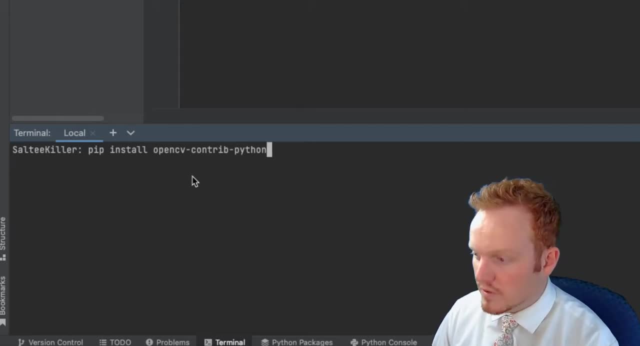 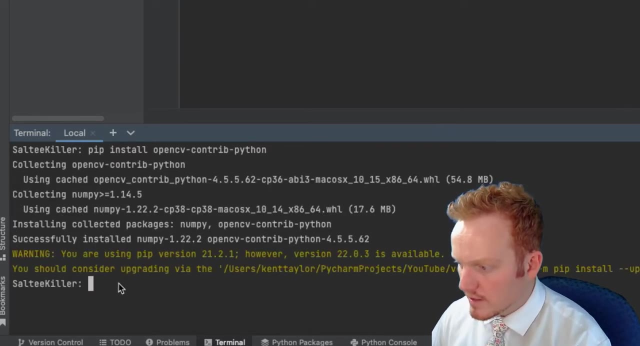 contain some extra libraries so that we have a little bit extra to work with. And so we're just going to hit enter and that's going to start installing. Okay, and if you ever get a warning, like I did, where you need to update pip or anything, you can go ahead and do that as well. 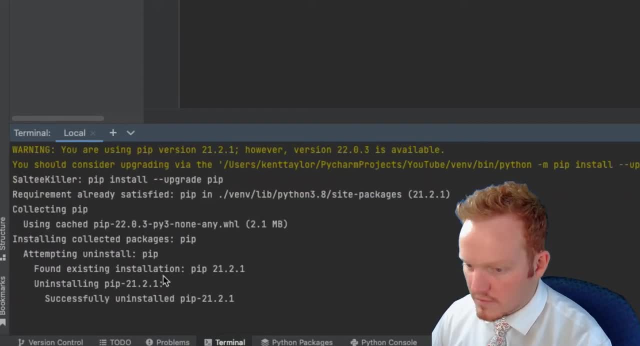 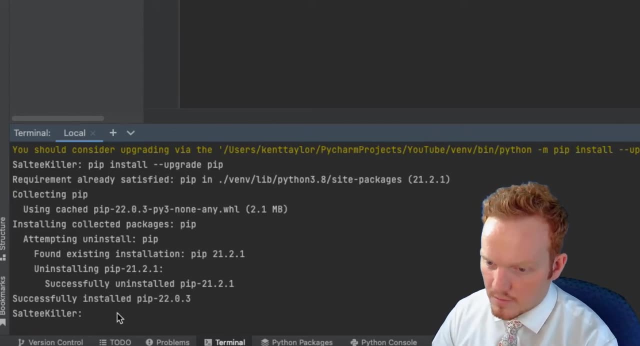 I'm just going to copy and paste that. That should be just really quick. And there we go, Perfect. After we have that installed, we are now going to go ahead and install C-Lib. So, pip, install cv lib. Okay, and we're going to be using this for our object detection. So there's a library. 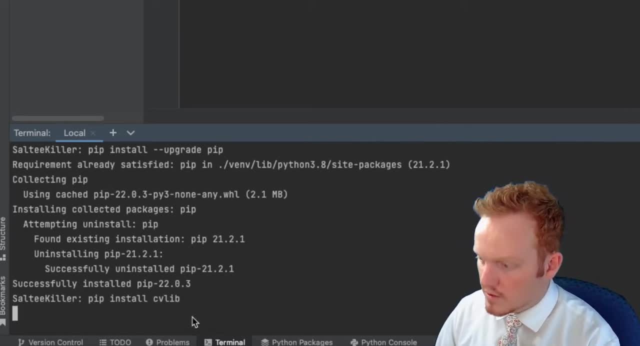 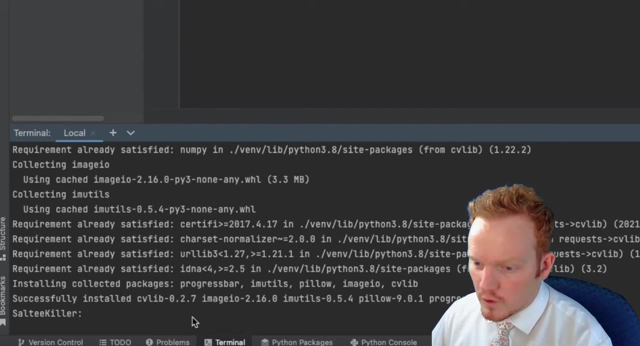 that's already learned what certain objects are. So we're just going to install that And depending on your internet connection, that should be rather quick, Very good. And then we're going to also allow our computer to say out loud what it saw. So if it sees me, it'll say: I saw a person. 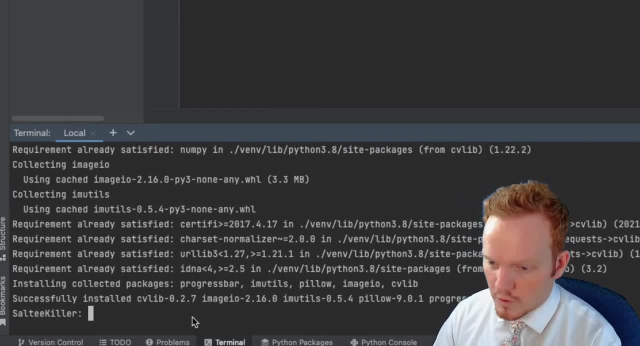 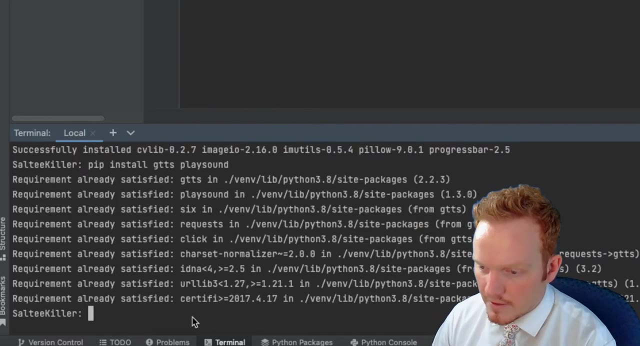 or I saw an apple, an orange, so on and so forth. We're going to import just a couple more things. We're going to say: pip, install gtts, space, play sound, Whoops, Play sound like that. And then, finally, we are going to install py. object C. 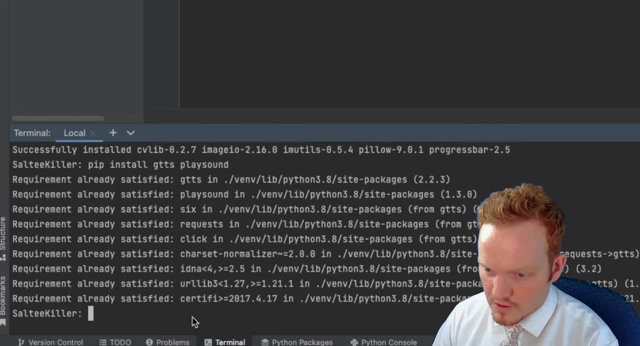 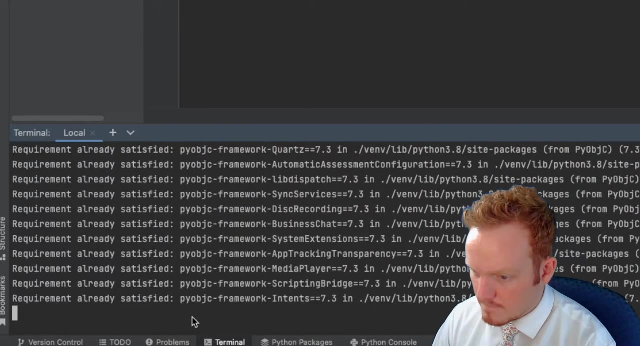 which is going to help with that sound be a little bit more efficient. So I'm going to say: pip three, install capital PY, capital O, B, J, capital C. Okay, so that will allow play sound to be a little bit more efficient. 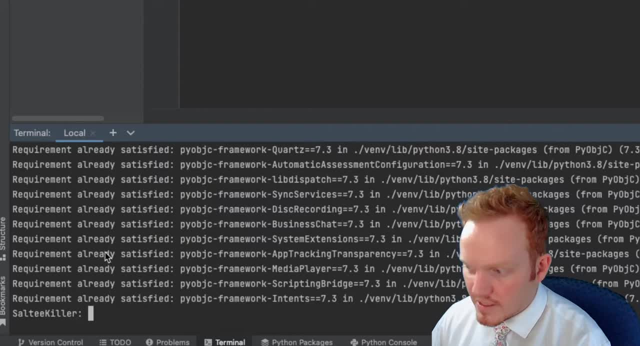 So I already have a couple of those installed. So it's going to say already satisfied For you. it will probably say successful. If you have any errors, just go back rewind. make sure that you typed everything correctly, Otherwise let's move on. So I'm just going to slide down my window here. 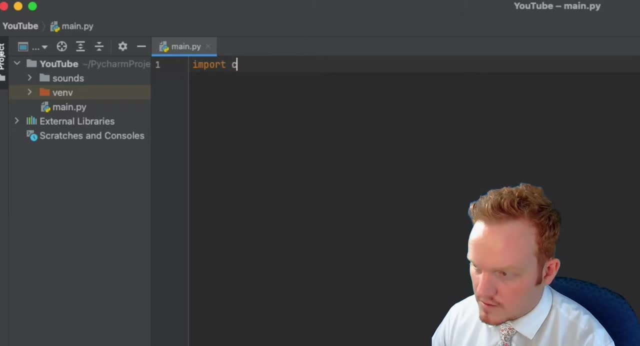 and I'm going to now import cv2.. import cv lib as cv And then from cv lib, dot, object detection. import draw box. So it's going to be drawing a box around our objects, for us. So make sure you have two B's for box, BBOX And then. 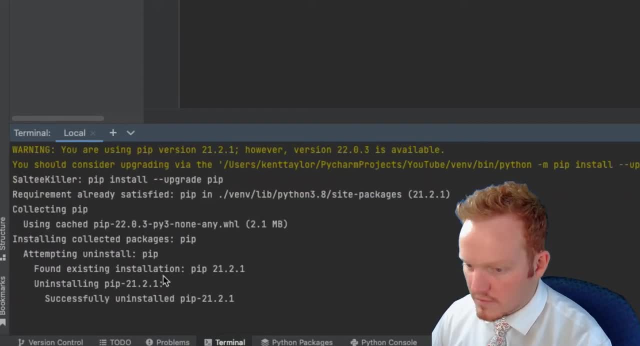 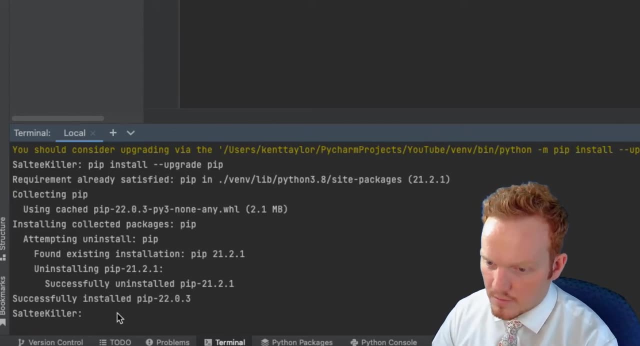 I'm just going to copy and paste that. That should be just really quick. And there we go, Perfect. After we have that installed, we are now going to go ahead and install C-Lib. So, pip, install cv lib. Okay, and we're going to be using this for our object detection. So there's a library. 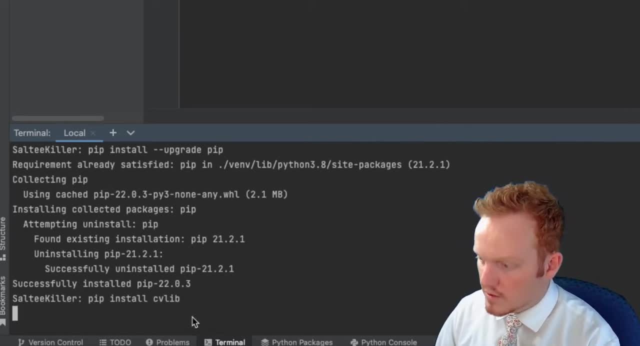 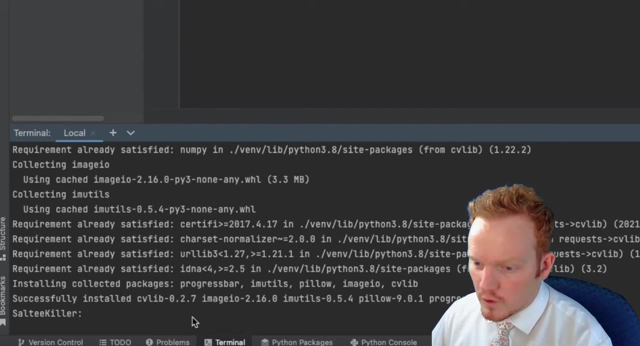 that's already learned what certain objects are. So we're just going to install that And depending on your internet connection, that should be rather quick, Very good. And then we're going to also allow our computer to say out loud what it saw. So if it sees me, it'll say: I saw a person. 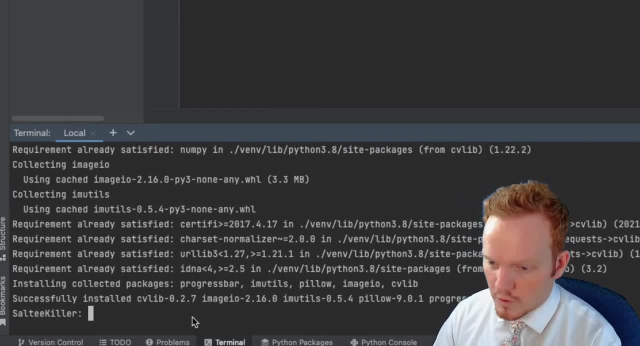 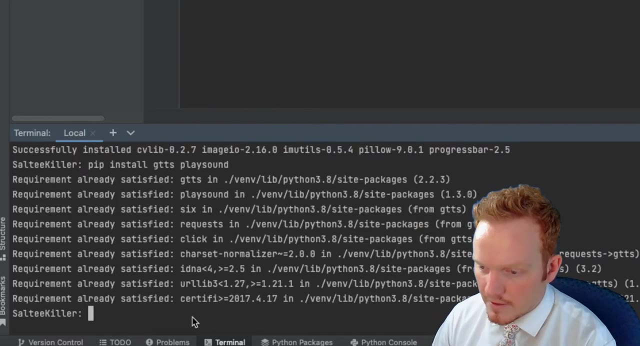 or I saw an apple, an orange, so on and so forth. We're going to import just a couple more things. We're going to say: pip, install gtts, space, play sound, Whoops, Play sound like that. And then, finally, we are going to install py. object C. 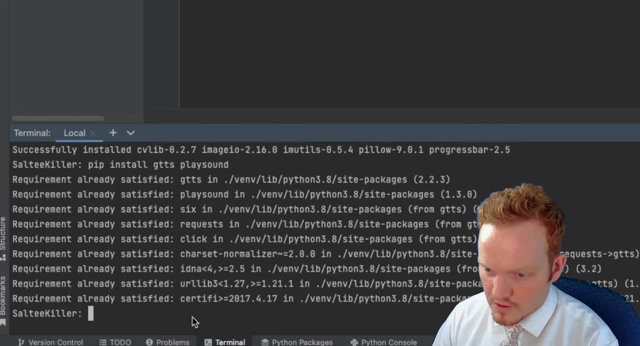 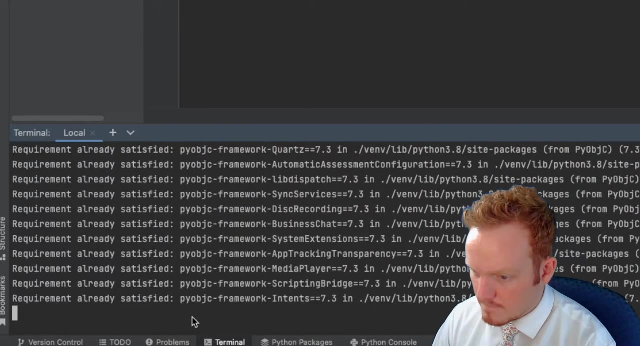 which is going to help with that sound be a little bit more efficient. So I'm going to say: pip three, install capital PY, capital O, B, J, capital C. Okay, so that will allow play sound to be a little bit more efficient. 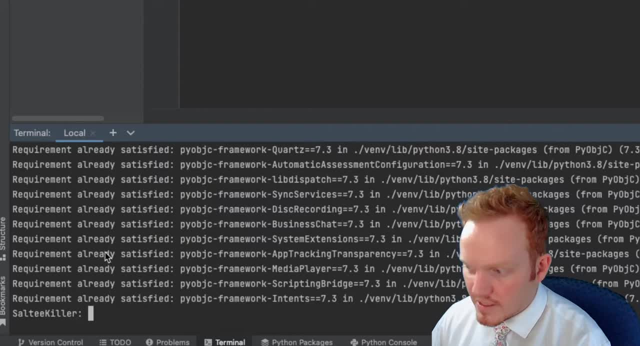 So I already have a couple of those installed. So it's going to say already satisfied For you. it will probably say successful. If you have any errors, just go back rewind. make sure that you typed everything correctly, Otherwise let's move on. So I'm just going to slide down my window here. 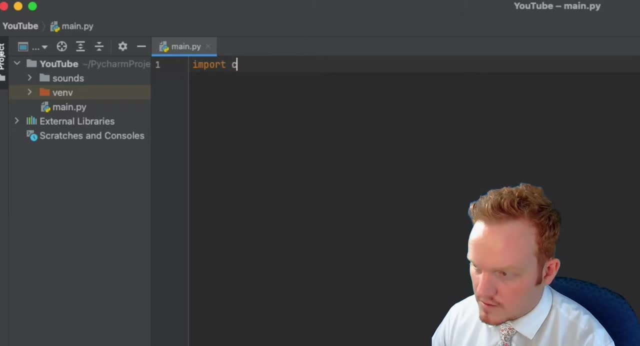 and I'm going to now import cv2.. import cv lib as cv And then from cv lib, dot, object detection. import draw box. So it's going to be drawing a box around our objects, for us. So make sure you have two B's for box, BBOX And then. 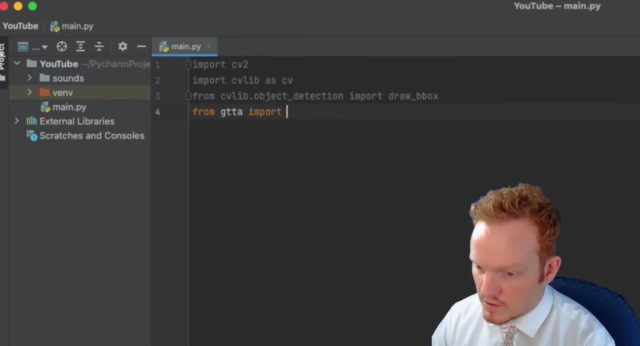 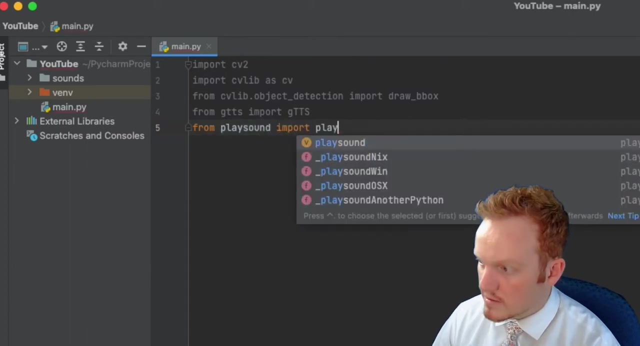 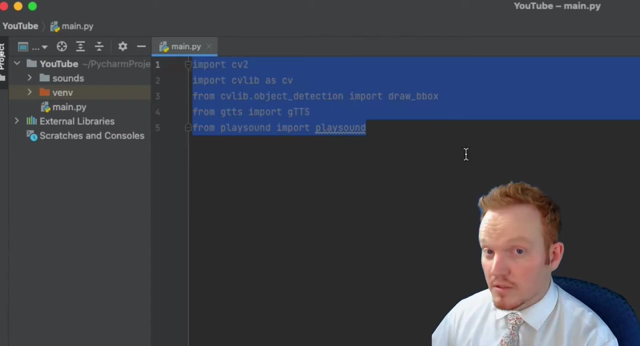 we're going to say: from gtts: import G capital, TTS. Oops, I said GTA, do gtts. Then finally, from play sound: import play sound. So there's 12345 lines of imports, But that is everything that we're going to be using for this. 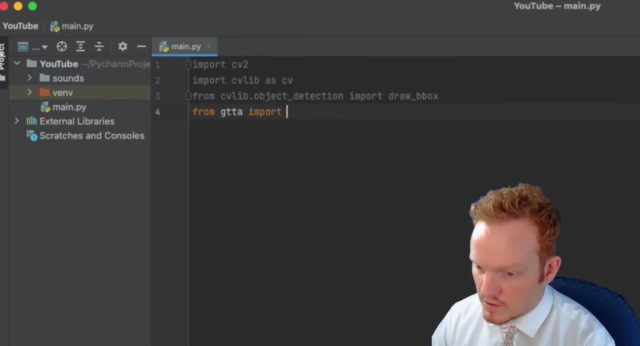 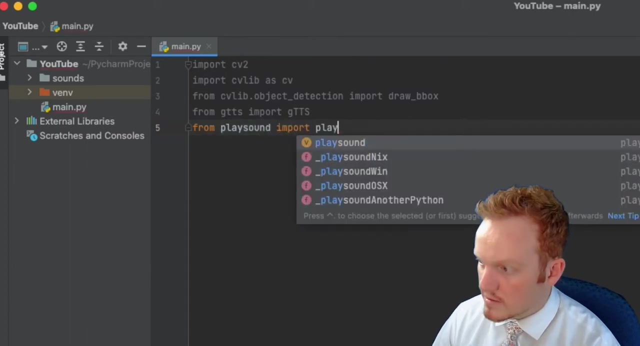 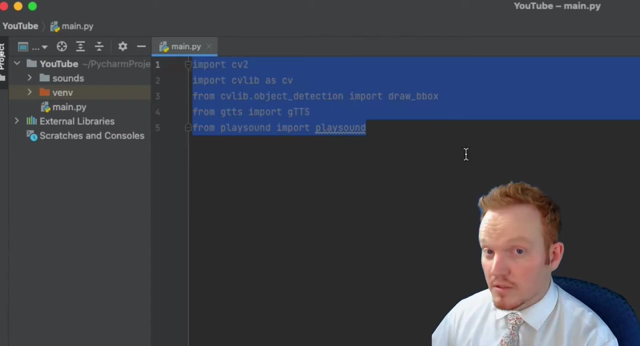 we're going to say: from gtts: import G capital, TTS. Oops, I said GTA, do gtts. Then finally, from play sound: import play sound. So there's 12345 lines of imports, But that is everything that we're going to be using for this. 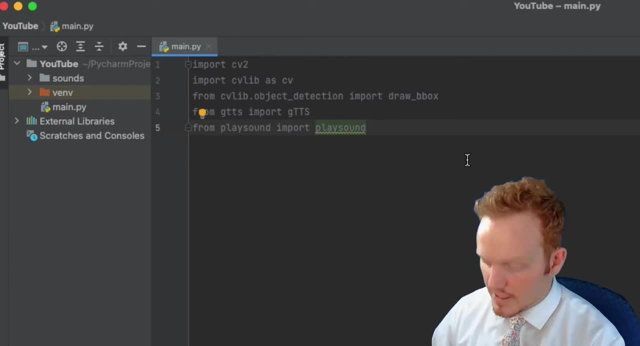 video. So if you need a little bit more time, you can go ahead and pause the video and continue that three days later. So what we want to do now is now access our camera Now- originally, when I was first building this and testing things out. 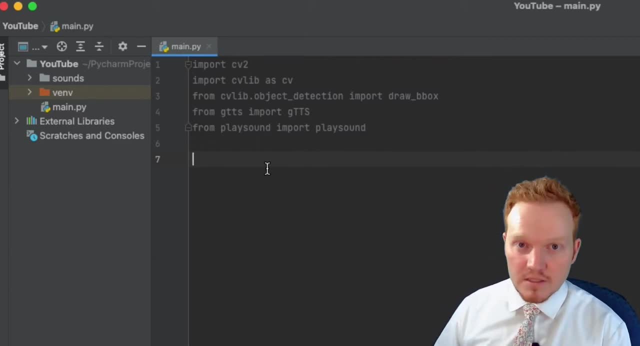 I was just having it bring in a specific image. I'm just going to look at objects in the image, But I wanted this to be live, So it has a live feed And we can detect all the objects in the live feed instead. So we're going to access our cameras. So I'm going to say video equals cv2 dot. 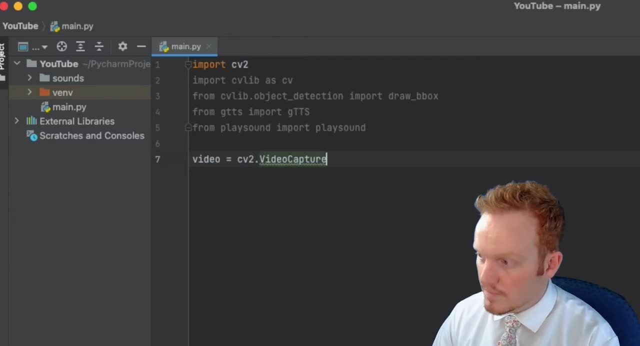 video Capture And that takes an index. Now, for most of you it might be index zero, but my web camera that I want to be using instead, which is a lot more higher quality, is that index one. So you can just mess with those indexes as you please, But we're going to start with that, And now we're. 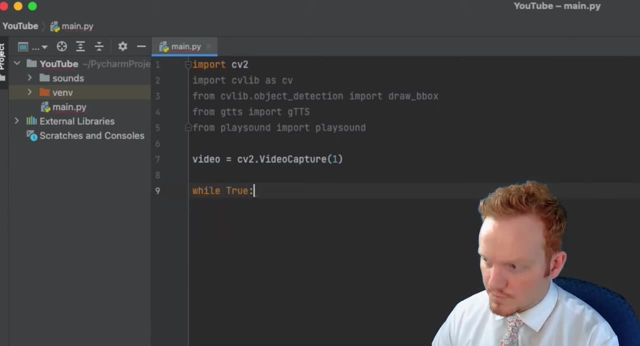 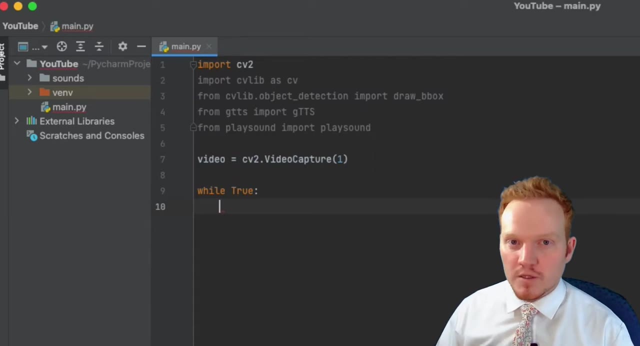 going to say: while: true, I'm now going to use my video capture And I'm going to unpack each frame into a variable called frame. So what we're going to do is: ret comma, frame equals our video dot read, So unpack that. So now we're going through each frame And now we're 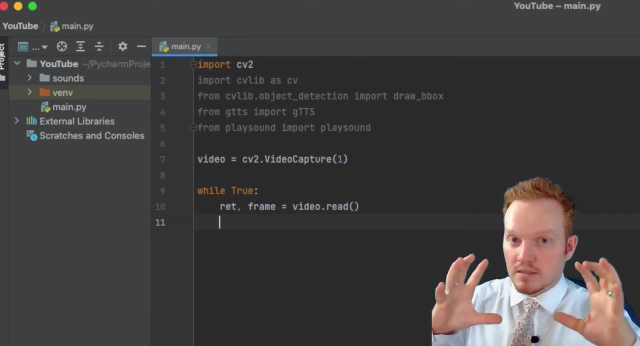 going to use that BB box where it's going to be seen the objects. it's going to draw a box around it And we're also going to give it a label next to the box to tell us what the object is. So we're 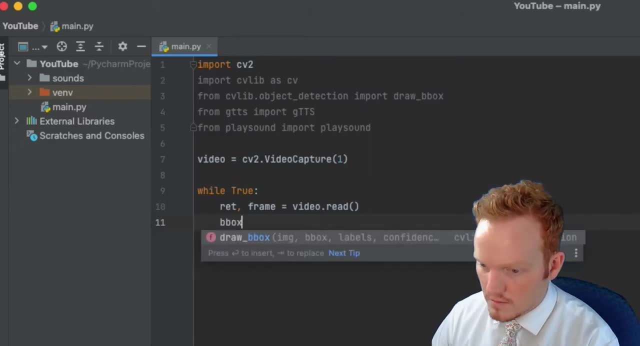 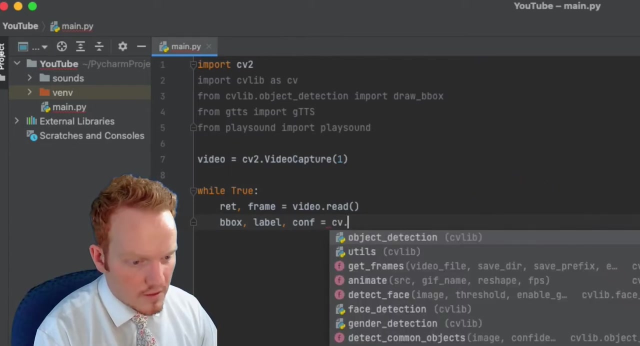 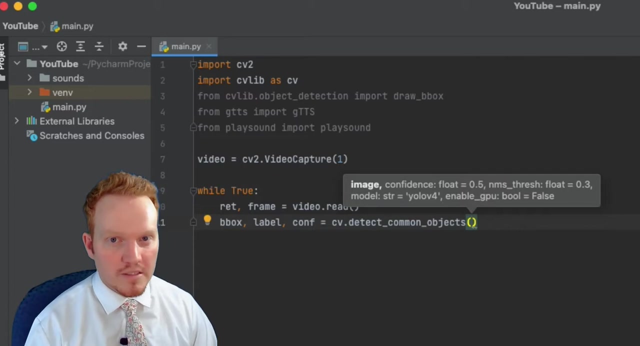 going to say BB box, comma label, And then comp, Okay, And comp is really just identifying what the object is. it's just going to be returning some decimal numbers, really. So I'm gonna say: cv dot detect common objects. And now we have to tell it where to get those objects from. So we need to say: 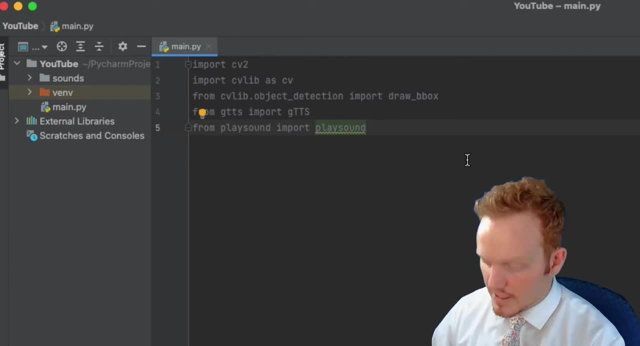 video. So if you need a little bit more time, you can go ahead and pause the video and continue that three days later. So what we want to do now is now access our camera Now- originally, when I was first building this and testing things out. 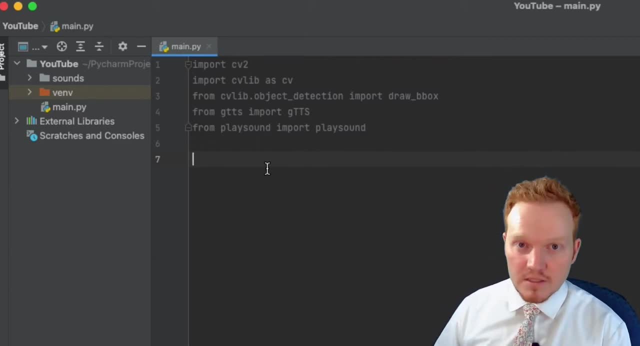 I was just having it bring in a specific image. I'm just going to look at objects in the image, But I wanted this to be live, So it has a live feed And we can detect all the objects in the live feed instead. So we're going to access our cameras. So I'm going to say video equals cv2 dot. 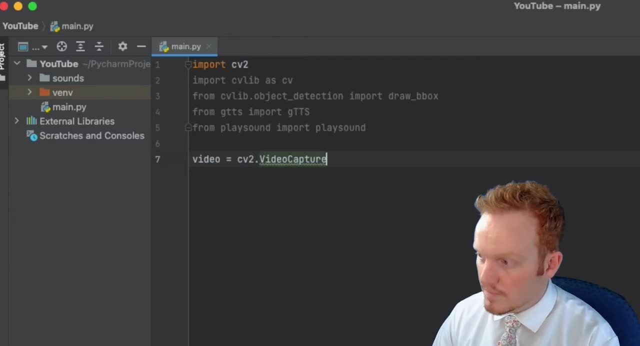 video Capture And that takes an index. Now, for most of you it might be index zero, but my web camera that I want to be using instead, which is a lot more higher quality, is that index one. So you can just mess with those indexes as you please, But we're going to start with that, And now we're. 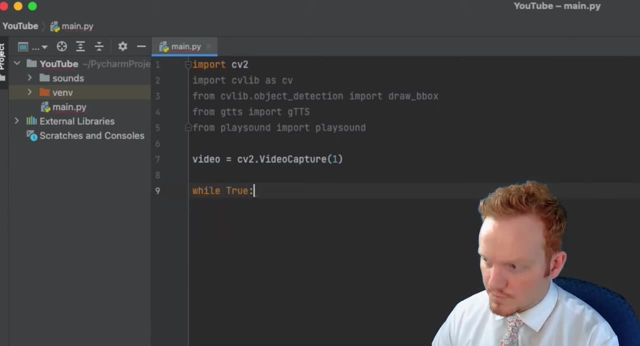 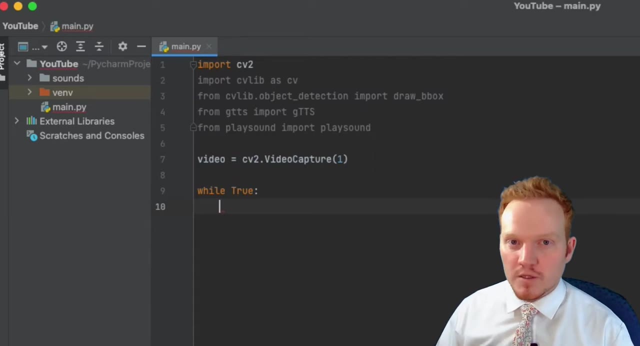 going to say: while: true, I'm now going to use my video capture And I'm going to unpack each frame into a variable called frame. So what we're going to do is: ret comma, frame equals our video dot read, So unpack that. So now we're going through each frame And now we're 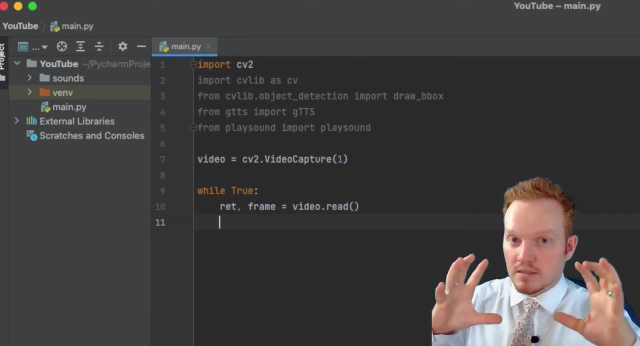 going to use that BB box where it's going to be seen the objects. it's going to draw a box around it And we're also going to give it a label next to the box to tell us what the object is. So we're 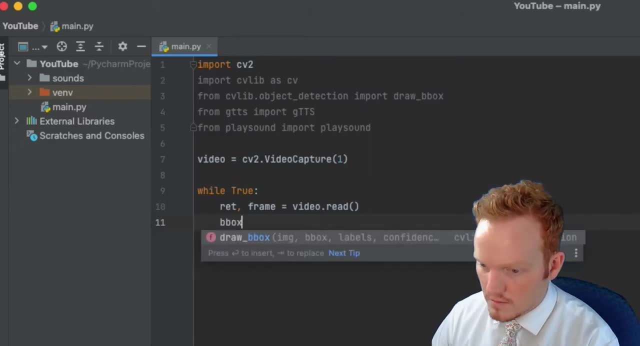 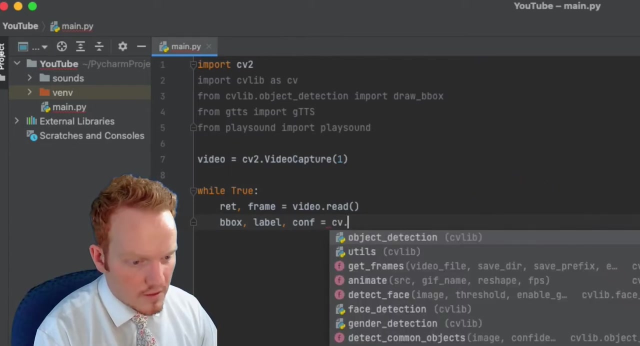 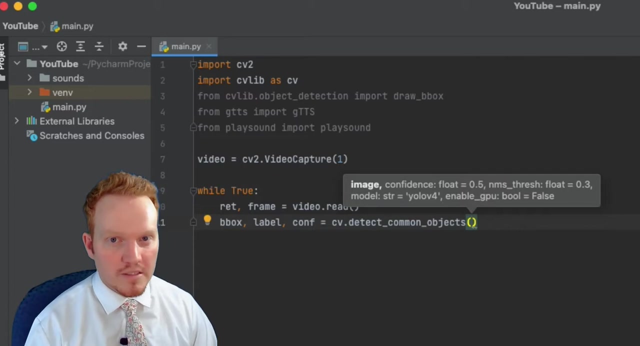 going to say BB box, comma label, And then comp, Okay, And comp is really just identifying what the object is. it's just going to be returning some decimal numbers, really. So I'm gonna say: cv dot detect common objects. And now we have to tell it where to get those objects from. So we need to say: 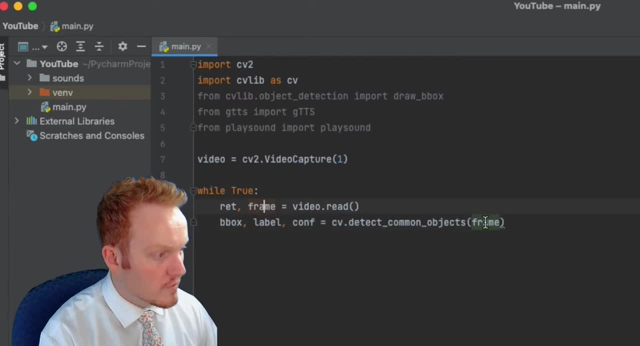 get it from the frame. So that's going to be each frame from my video feed. And finally, we are going to draw that box. So we're going to say output image equals draw box. And now we need to give draw box the frame. 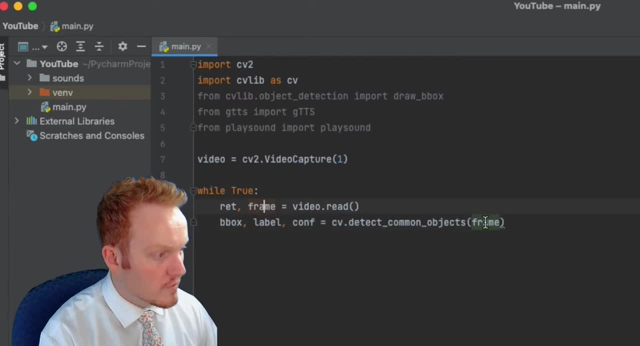 get it from the frame. So that's going to be each frame from my video feed. And finally, we are going to draw that box. So we're going to say output image equals draw box. And now we need to give draw box the frame. 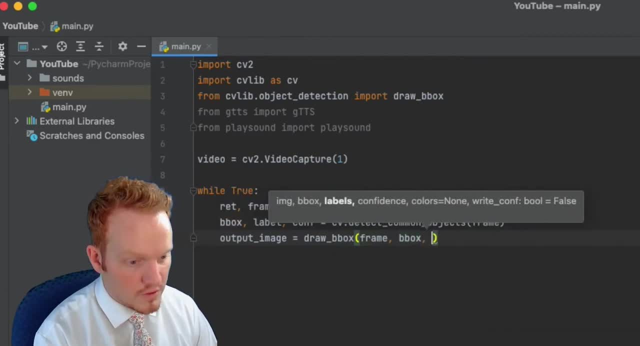 I want it to get the box that it's going to be drawing around, And we're also going to put the label in there And we'll stick conf in there, Very good, So now that we have that, let's go ahead and show the user what they're going to see. So let's go ahead and show the user what they're. 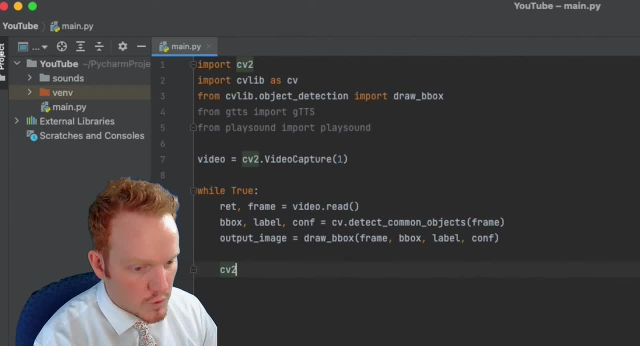 image looks like. So I'm going to say cv, two dot, I am show, And we want to show them the name of the window. So I'll just call this object detection. you can call that whatever you want- comma. And now we've got to tell it output image. Okay, before we hit run, we're going to 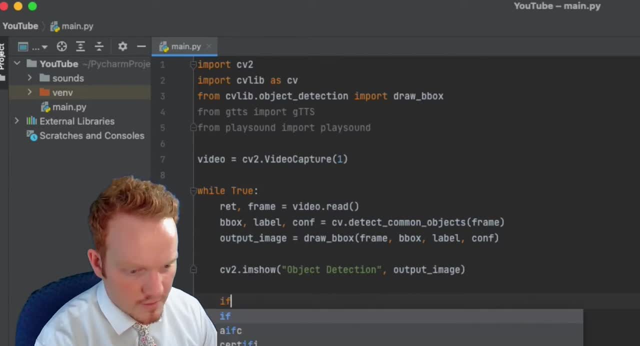 give this a weight key. So I'm going to say if cv two dot weight key, delay of one and we're going to check to see if the user is clicking a certain button, You can say whatever button you want, But I'm going to say if the user 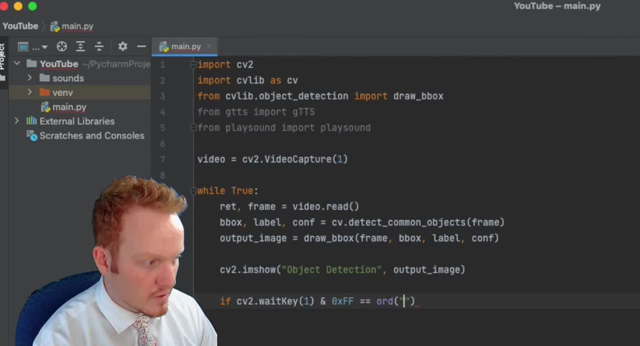 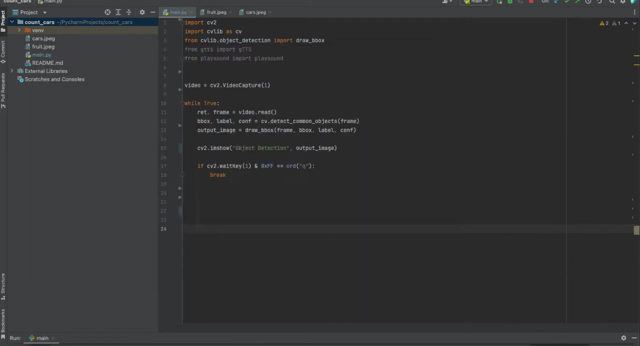 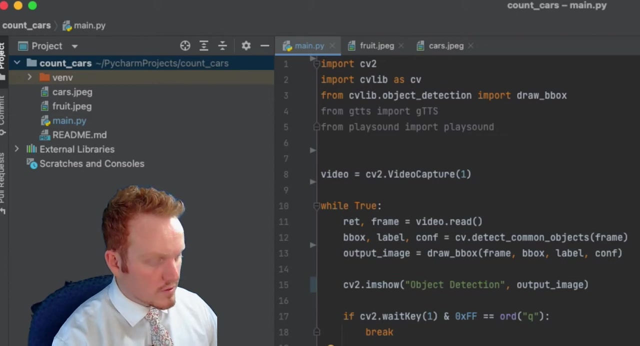 clicks on Q- some people like the spacebar. you can just do a space, do whatever you want. But I'm gonna say, if the user says hits Q, I want you to break out of this loop. And after I hit Q, it breaks out of that window. So very good. So, as you can see, that was already. 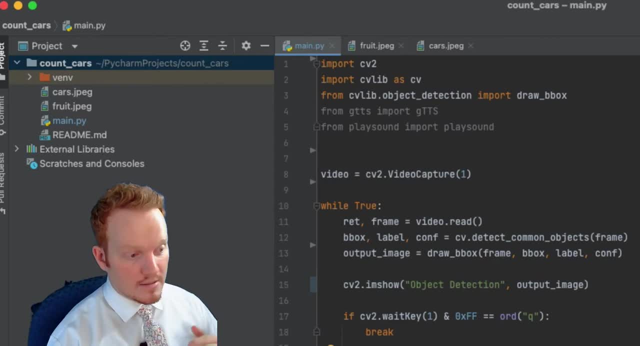 detecting me as a person, even detected this as a tie. that's already working. So what I want this to do now is I want my program to take each of those labels that it finds in my screen and I want it to append or add to a list so that I have that list of data. So what we're going to do now 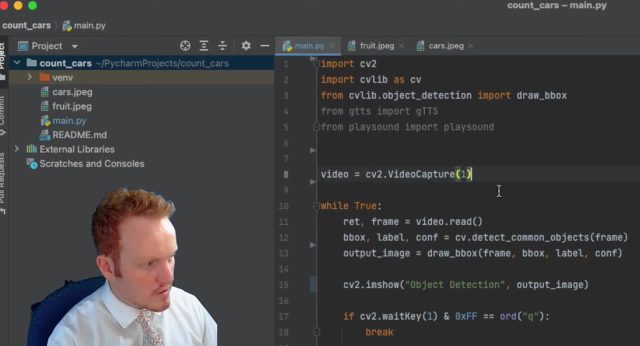 is: we're going to make a list of data. So we're going to make a list of data, So we're going to call it labels. So let's come up here and we'll call this labels. Make sure this is outside of. 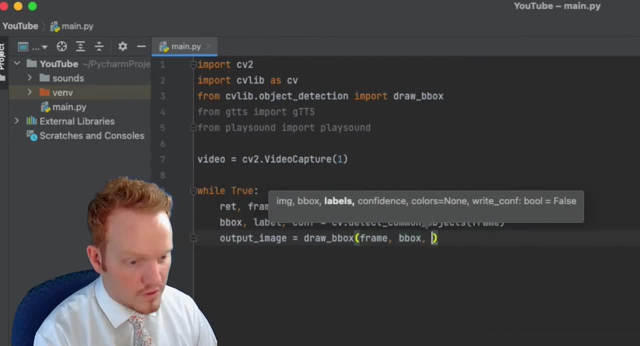 I want it to get the box that it's going to be drawing around, And we're also going to put the label in there And we'll stick conf in there, Very good, So now that we have that, let's go ahead and show the user what they're going to see. So let's go ahead and show the user what they're. 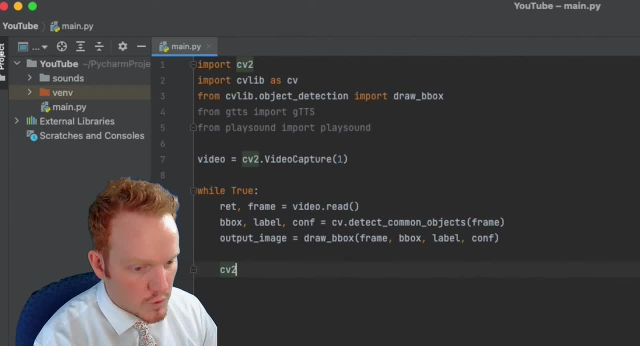 image looks like. So I'm going to say cv, two dot, I am show, And we want to show them the name of the window. So I'll just call this object detection. you can call that whatever you want- comma. And now we've got to tell it output image. Okay, before we hit run, we're going to 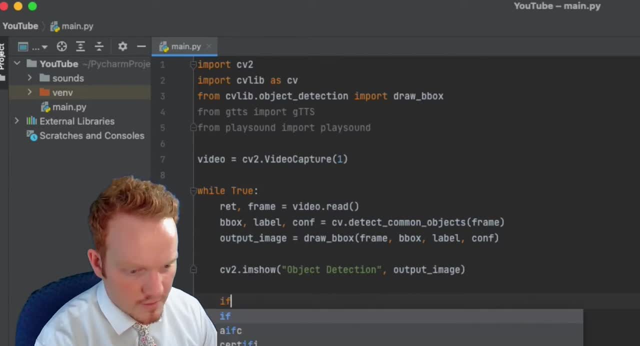 give this a weight key. So I'm going to say if cv two dot weight key, delay of one and we're going to check to see if the user is clicking a certain button, You can say whatever button you want, But I'm going to say if the user 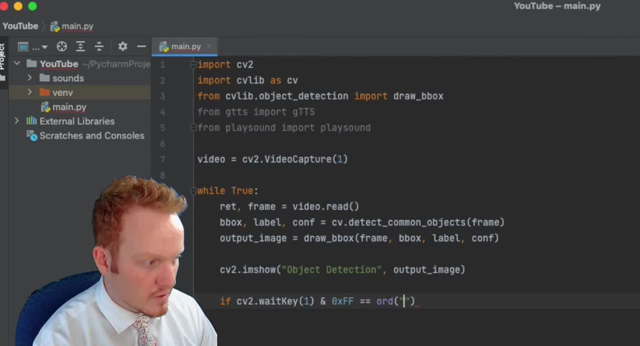 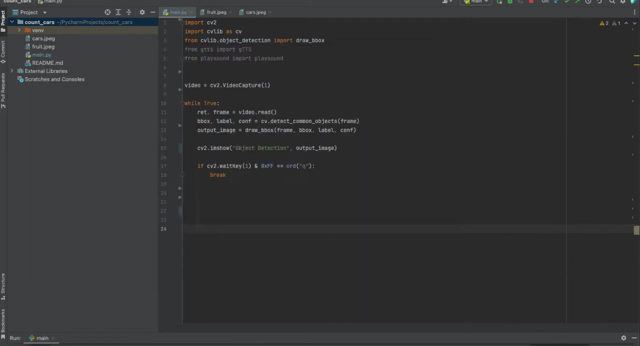 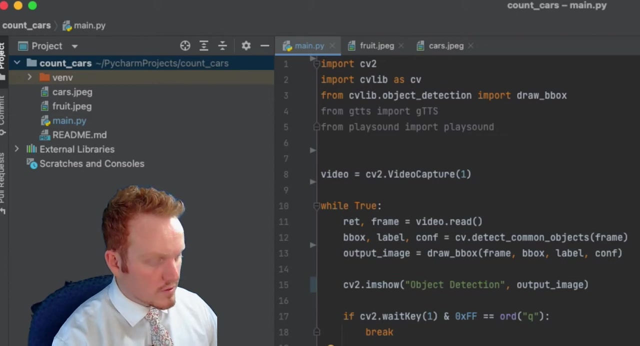 clicks on Q. some people like the space bar. you can just do a space, do whatever you want, But I'm going to say, if the user says hits Q, I want you to break out of this loop. And after I hit Q, it breaks out of that window. So very good. So, as you can see, that was already. 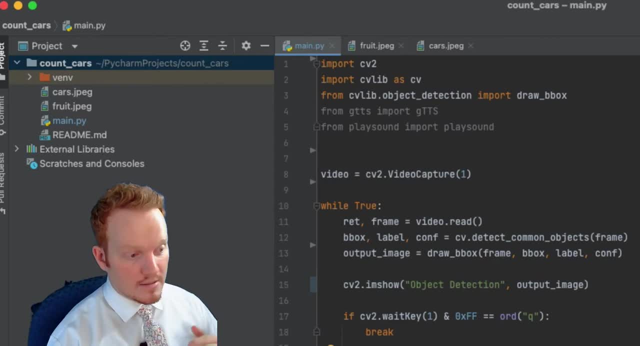 detecting me as a person, even detected this as a tie. that's already working. So what I want this to do now is I want my program to take each of those labels that it finds in my screen and I want it to append or add to a list so that I have that list of data. So what we're going to do now 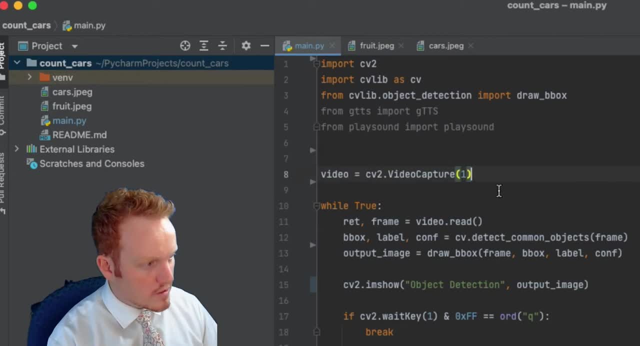 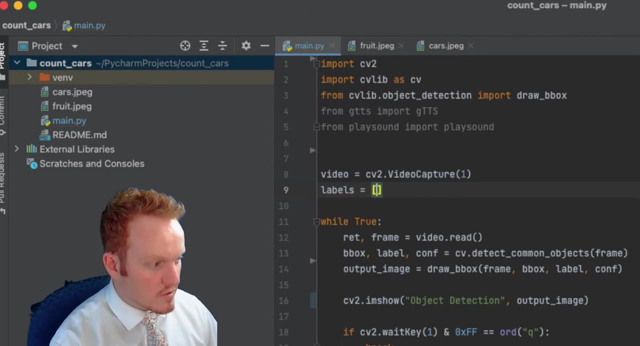 is, we're going to make a list of data, So we're going to make a list of data, So we're going to call this labels. So let's come up here And we'll call this labels. Make sure this is outside of your loop So it doesn't accidentally rename itself inside the loop and just erase all the. 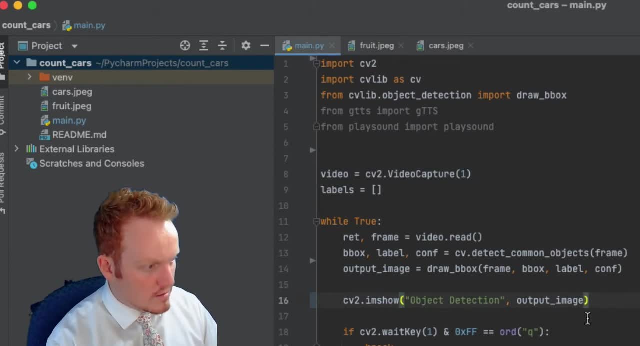 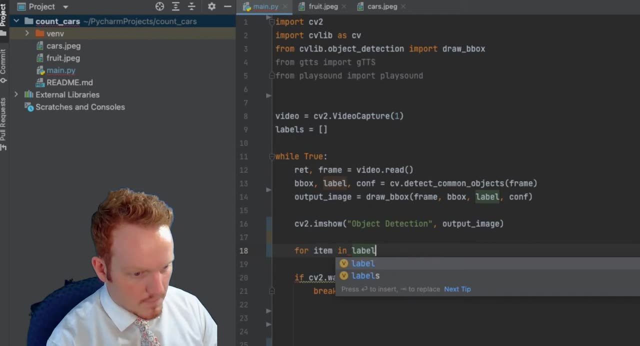 data And what we're going to say is we'll do a for loop. we're going to say, for item in label, If item in labels, then we're just going to have it pass. So that means if, if it already found a tie, this is going to be checking multiple images. 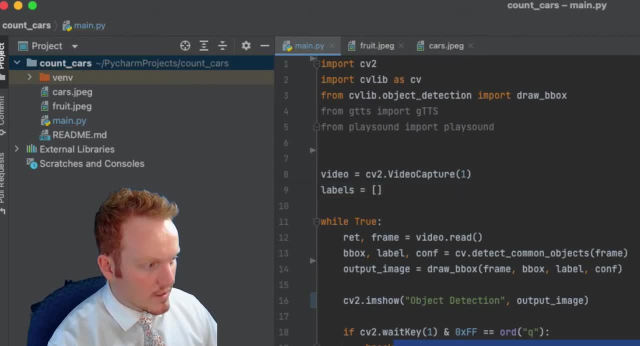 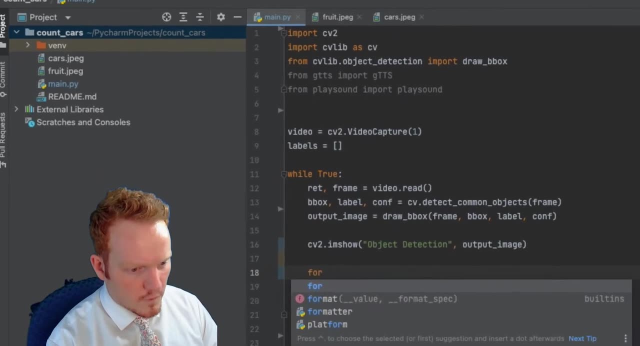 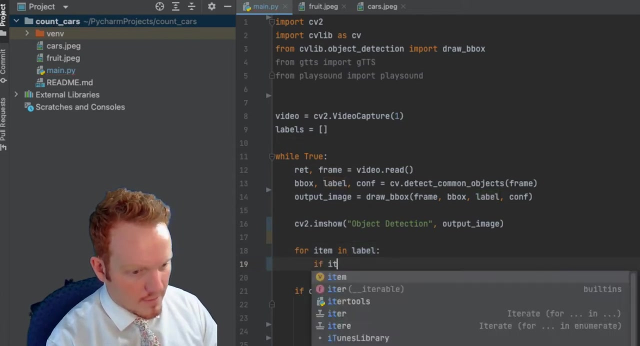 your loop So it doesn't accidentally rename itself inside the loop and just erase all the data. And what we're going to say is we'll do a for loop. we're going to say for item in label, If item in labels. 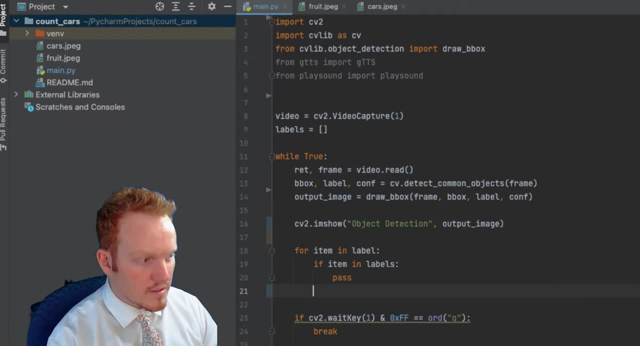 then we're just going to have it pass. So that means if- if it already found a tie- this is going to be checking multiple images, it's going to be checking for objects in each frame, And so it's going to say maybe like 1000. 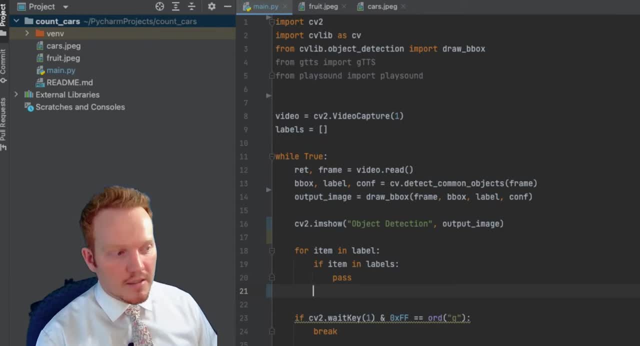 ties. I don't want it to do that. I'm just going to say if you find a tie in there, then go ahead and put it in the list. But ties are already in the list, don't add it to the list. So it's only. 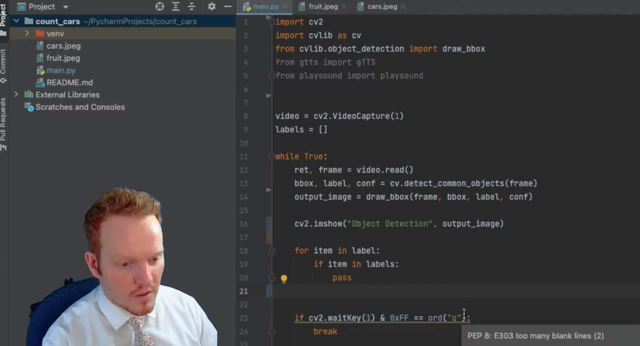 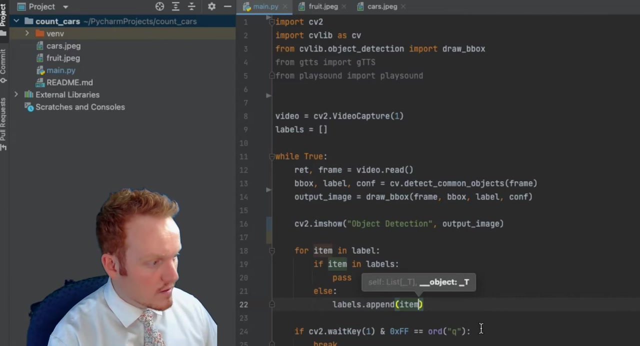 going to say tie one time And you can alter this if you'd like, But this is the way I'm going to do it. If it's not already in the list, then I want you to labels dot append. I want you to append that item So that item will be added to this list called labels. And just to test that. 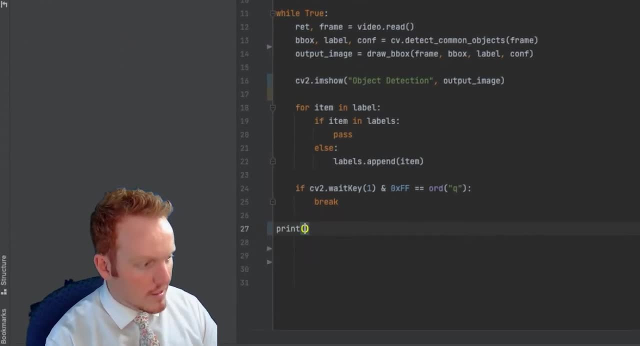 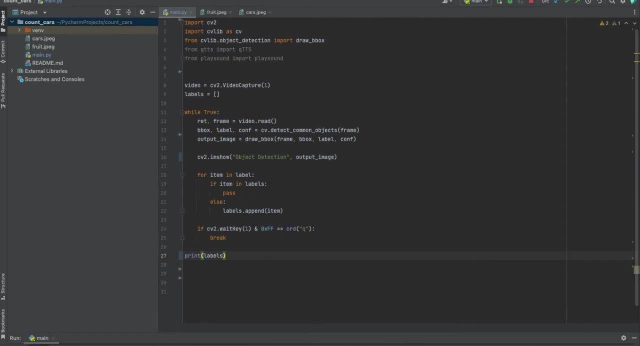 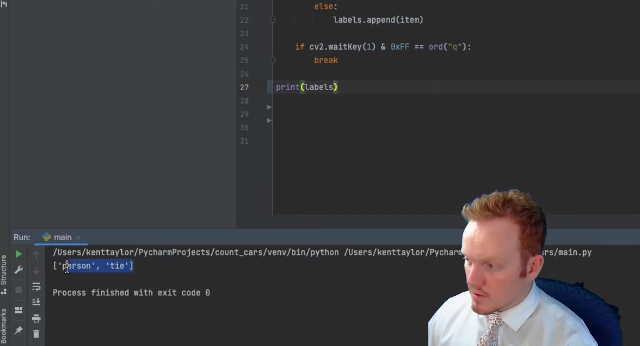 out. I'm going to come down here and print labels And let's see if that works. Okay, and, as you can see, here is my list called labels that it just printed. So it found a person and it found a tie. So very good, I know that this is working, because if I didn't, 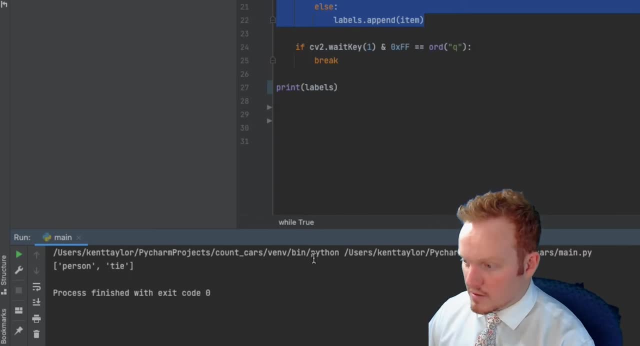 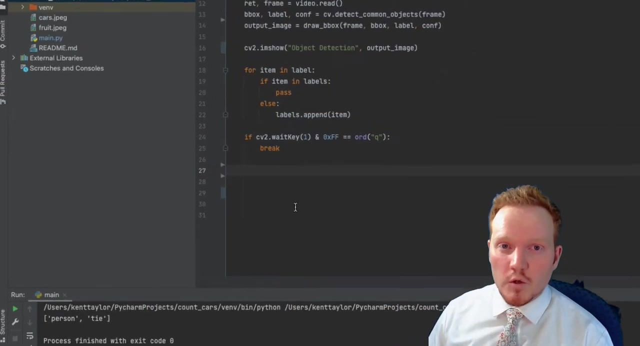 it would be saying person 1000 times in the tie 1000 times, but it's only going to do it once because of this code here. So very good. So what I want this to do now is: I wanted to take this data called labels, So what I'm going to do now is write code using string interpolation to tell: 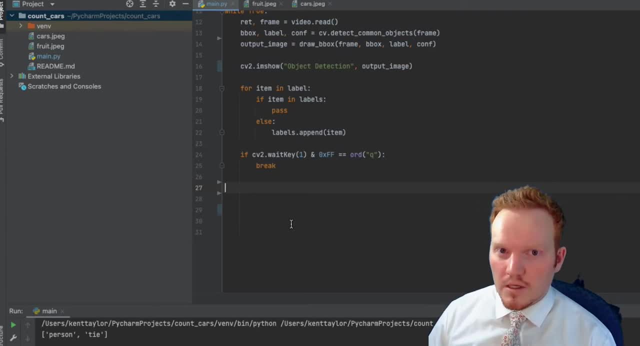 me what it found more logically. For example, I wanted to say something like: I found an orange, a person, a book, a tie, a cell phone, an apple, so on and so forth. And so how I'm going to do, 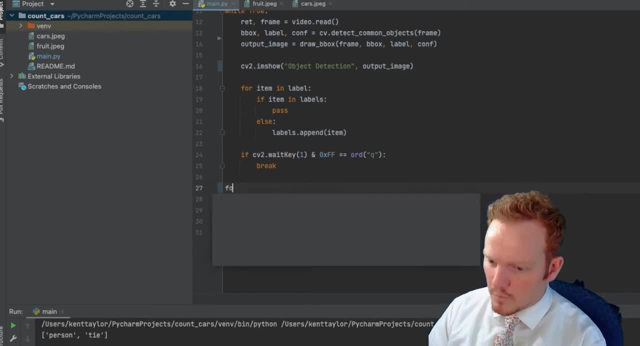 that is, I'm going to create a for loop for label in labels. So I'm going to create a for loop for label in labels. I want this to be a label, So I'm going to create a for loop for label in labels. 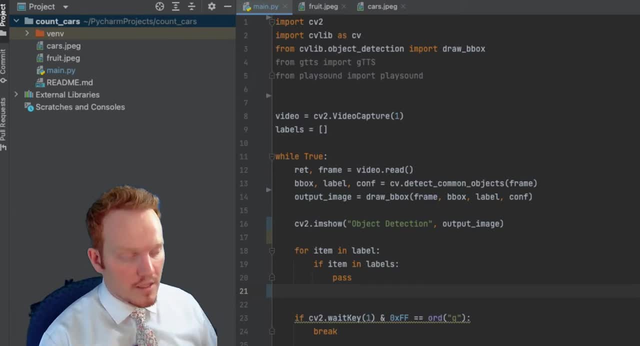 it's going to be checking for objects in each frame And so it's going to say, maybe like 1000 ties. I don't want it to do that. I'm just going to say if you find a tie in there, then go ahead. 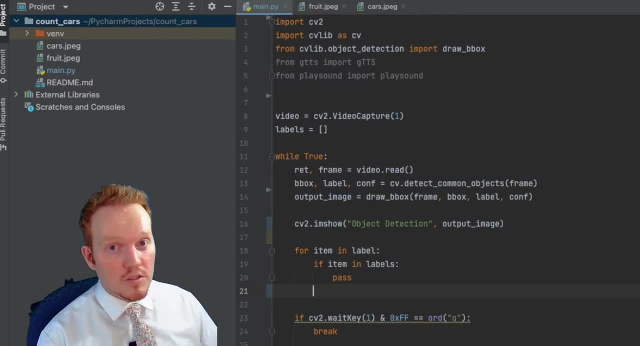 and put it in the list. But ties are already in the list, don't add it to the list. So it's only going to say tie one time And you can alter this if you'd like, But this is the way I'm. 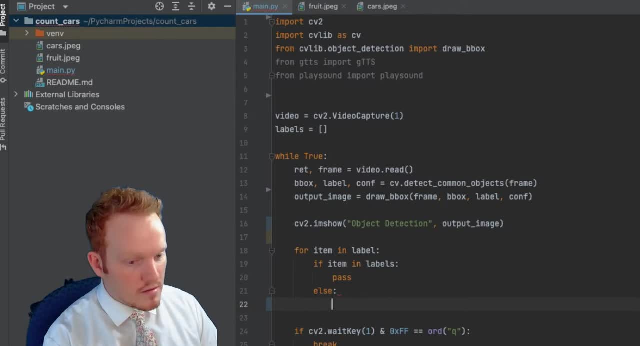 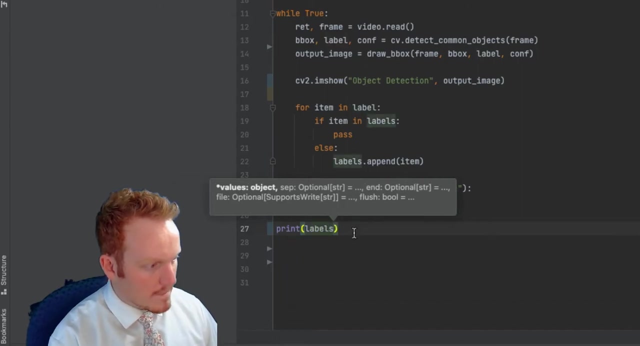 going to do it. If it's not already in the list, then I want you to labels dot append. I want you to append that item So that item will be added to this list called labels. And just to test that out, I'm going to come down here and print labels And let's see if that works. 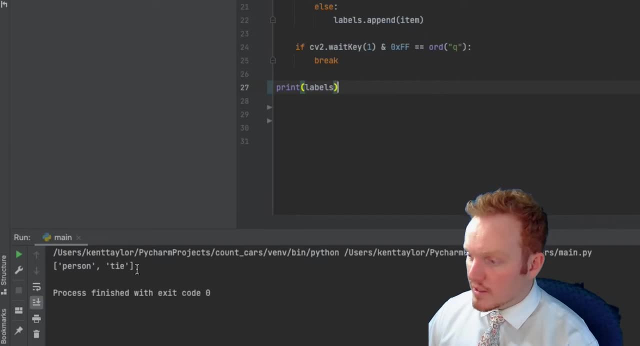 Okay, and, as you can see, here is my list called labels that it just printed. So it found a person and it found a tie. So, very good, I know that this is working, because if I didn't, it would be saying person 1000 times in the tie 1000 times, but it's only going to do it once. 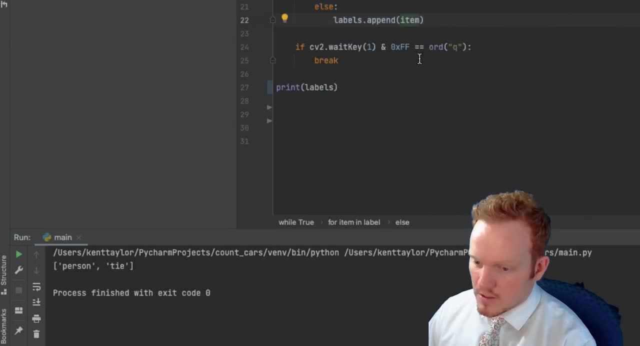 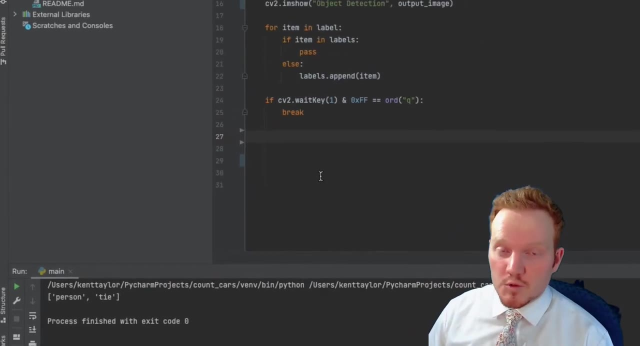 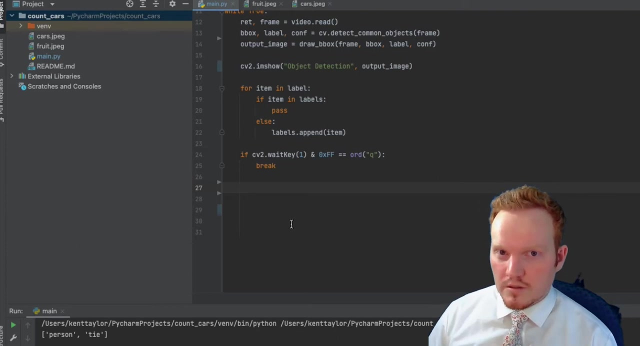 because of this code here. So very good. So what I want this to do now is: I wanted to take this data called labels. So what I'm going to do now is write code using string interpolation to tell me what it found more logically. For example, I wanted to say something like I found an orange. 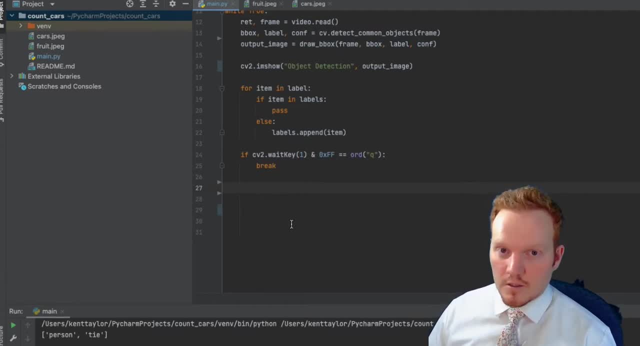 a person, a book, a tie, a cell phone, an apple, so on and so forth. And so how I'm going to do that is I'm going to create a for loop for label in labels. So I'm going to create a for loop for label in labels. 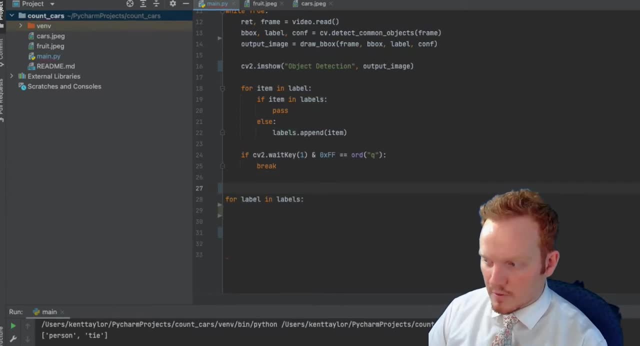 I want this to be a label. So I'm going to create a for loop for label in labels to check to see if this is the first time it's reading out loud a label. So I'm going to create some kind of iterator. So I'm going to say I equals zero And I'm going to say here, if I 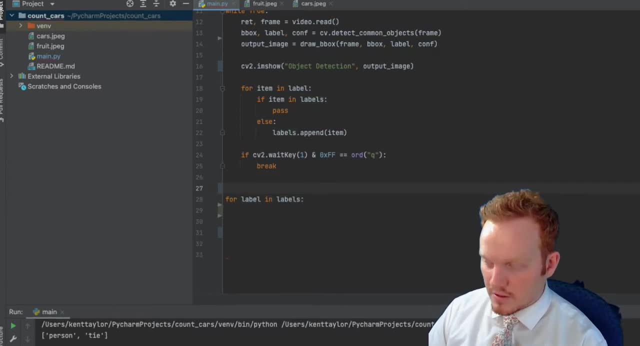 So I'm going to create a for loop for label in labels. So I want this to check to see if this is the first time it's reading out loud a label. So I'm going to create some kind of iterator. So I'm going to say I equals zero And I'm going to say here, if I is zero, then I want this to actually. 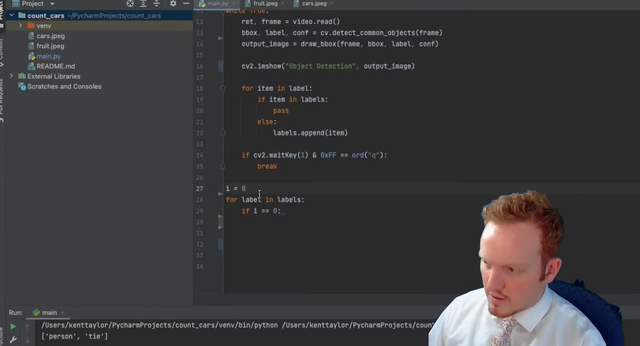 append to a list. So I want this to sound a little bit more natural when it says it out loud. So I'm going to say new sentence equals an empty list. So I'm going to say if I is zero, then new sentence dot. append that means to add, and I want it to add. I'll use some string interpolation. 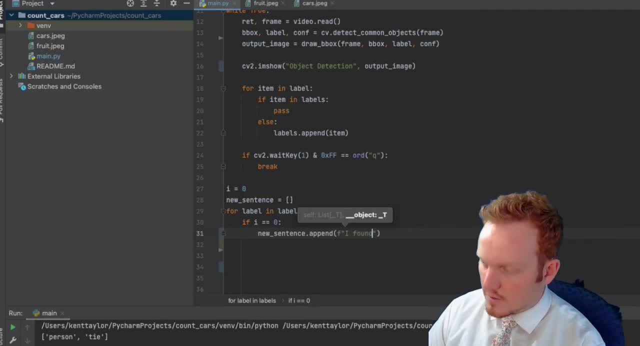 here I found a. I'll put label there. So if it's found a person, I'll say I found a person And I'll do a comma and comma. They'll give this speech out loud to give a little bit of a pause. 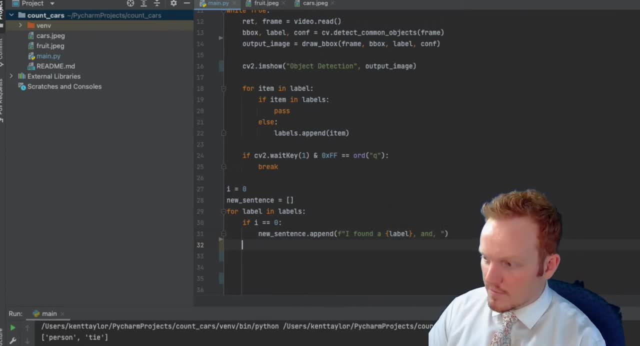 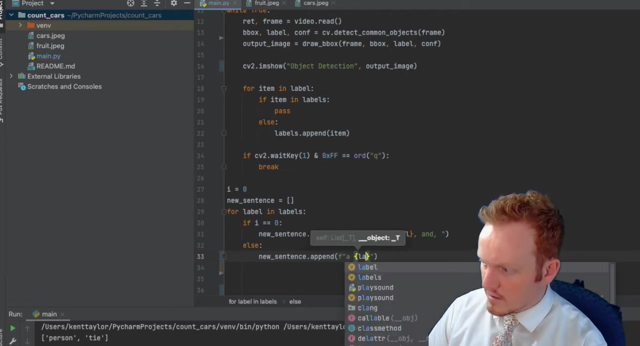 So we'll see how that goes. And then I'm going to say: if it is not equal to zero, then new sentence, dot append, and I'll use string interpolation again And I'm going to say a label like so, And then once that is done, we are going. 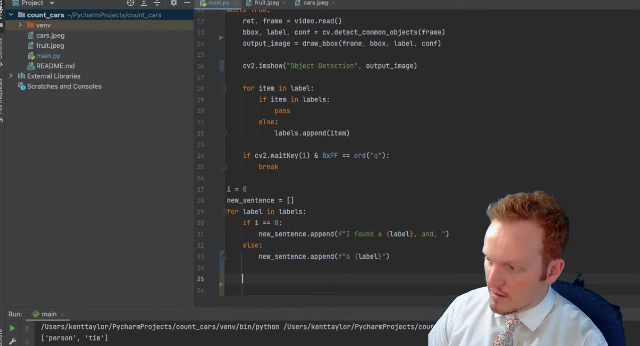 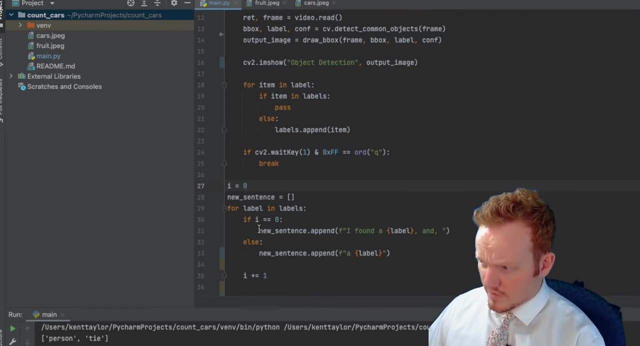 to increment I. so I'm going to say I plus equals one. So the first thing it finds I is it can be zero. So the first thing it finds is going to say I found a person. So I'm going to say I found a. 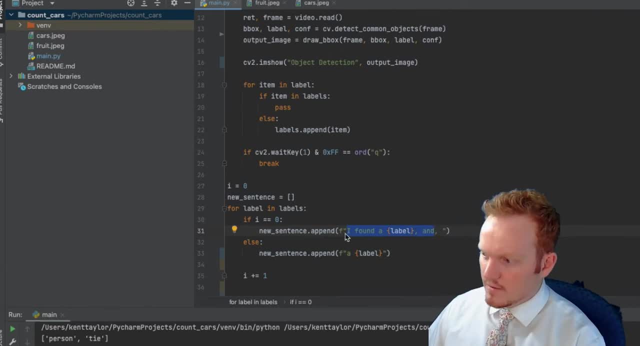 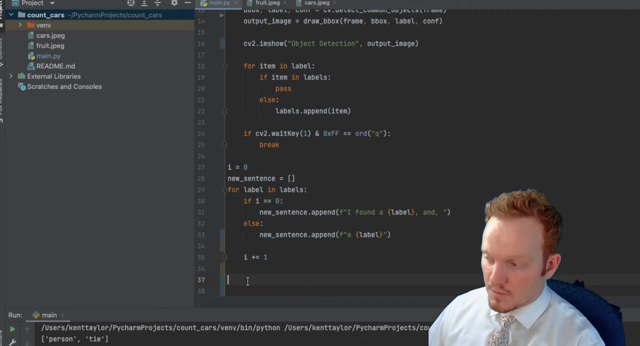 hat and a person, a book, an apple, so on and so forth. So very good with that, And just to make sure that this is all going to be all in one string for our speech to work properly, After this, let's go ahead and use the join function. So I'm just going to say print space, dot, join. 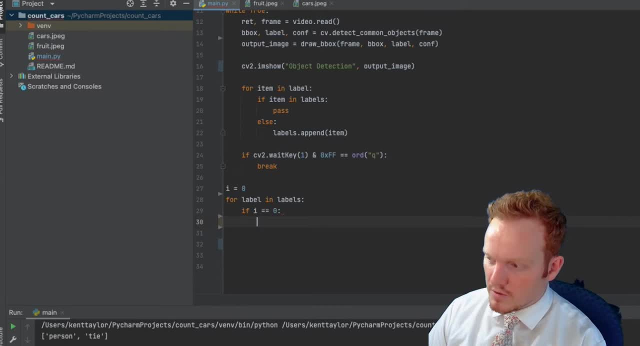 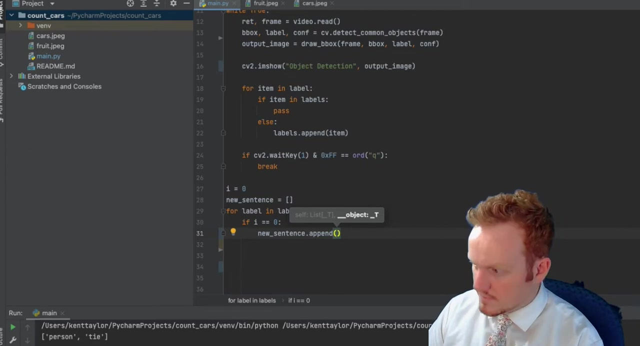 zero. then I want this to actually append to a list. So I want this to sound a little bit more natural when it says it out loud. So I'm gonna say: new sentence equals an empty list. So I'm going to say: new sentence dot. append, That means to add, and I want it to add. I'll use some string. 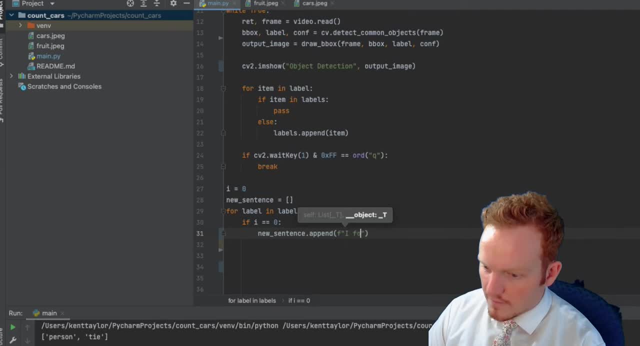 interpolation. here I found a, I'll put label there. So if it found a person, I'll say I found a person And I'll do a comma and comma. I'll give this speech out loud to give a little bit of a. 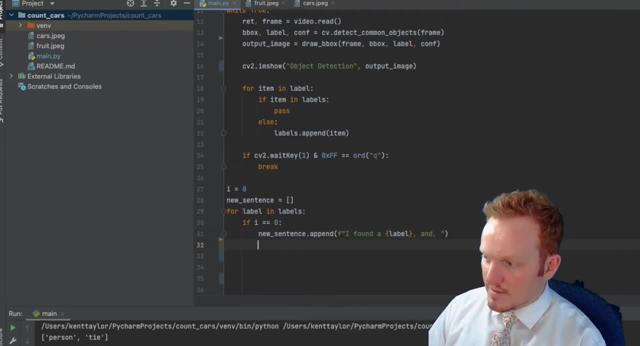 pause, So we'll see how that goes. And then I'm going to say: I found a person And I'll do a comma and comma. And then I'm going to say: if it is not equal to zero, then new sentence dot. 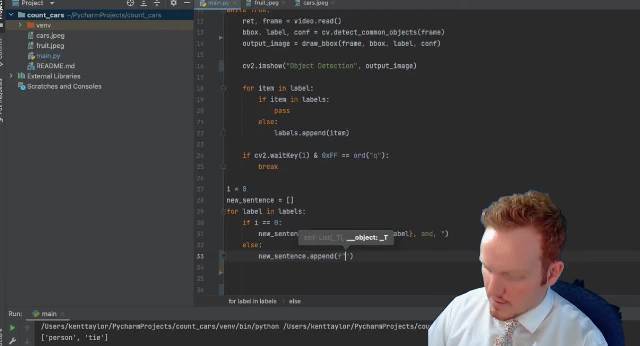 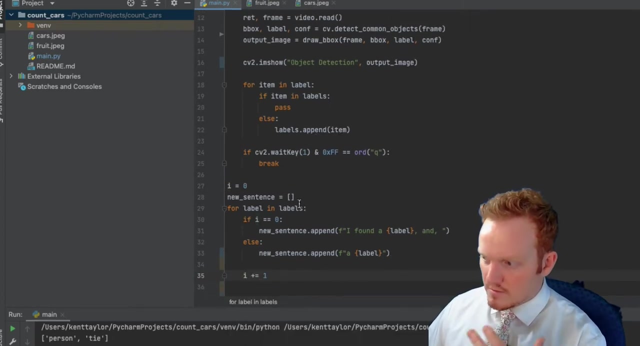 append And I'll use string interpolation again And I'm going to say a label like so, And then, once that is done, we are going to increment I. So I'm going to say I plus equals one. So the first thing it finds I is going to be zero. So the first thing it finds is going to say I found a. 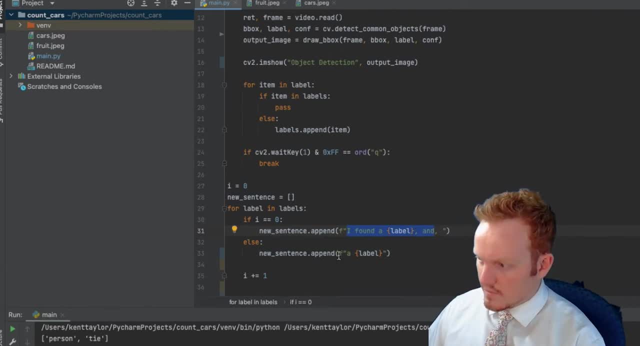 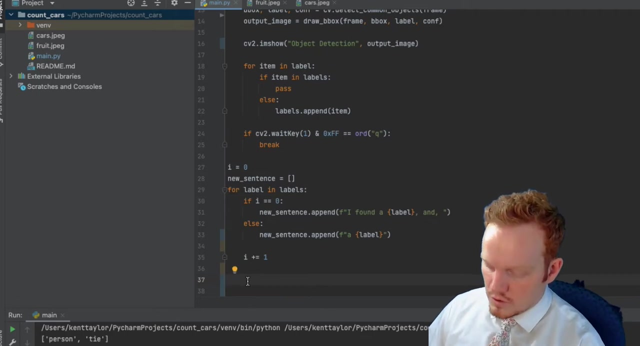 hat and a person, a book, an apple, so on and so forth. So very good with that, And just to make sure that this is all going to be all in one string for our speech to work properly after this, let's go ahead and use the join function. So I'm just going to say: print space dot, join new sentence. 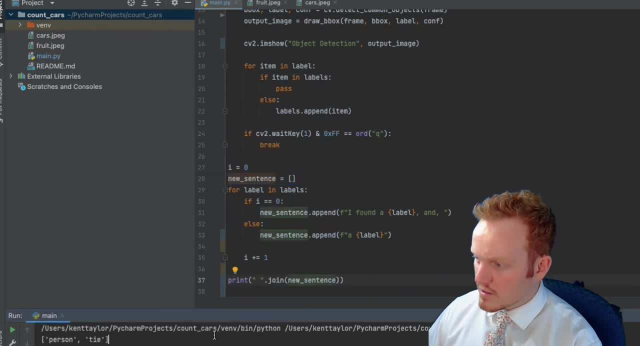 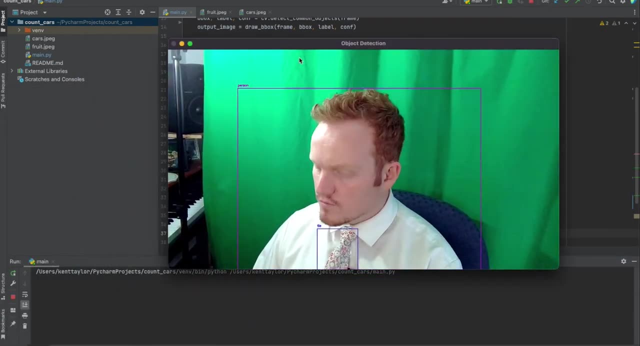 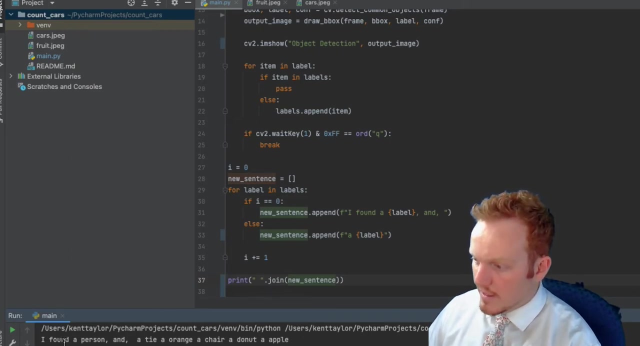 So that will turn this list into a string. So let's go ahead and test that out. Perfect. So after hitting run and after it found those things, check it out. It added each of those things to the list. So it said I found a person and a tie. 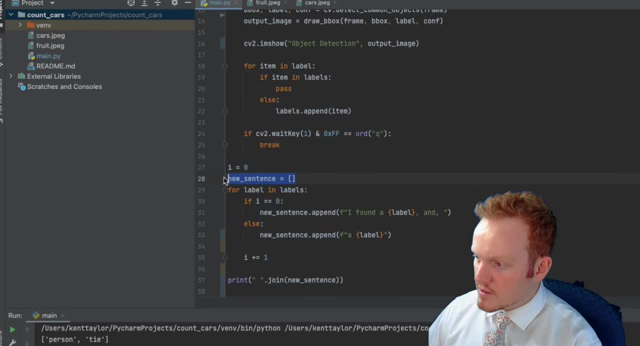 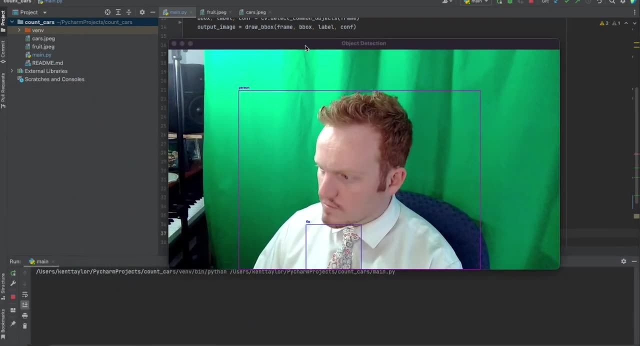 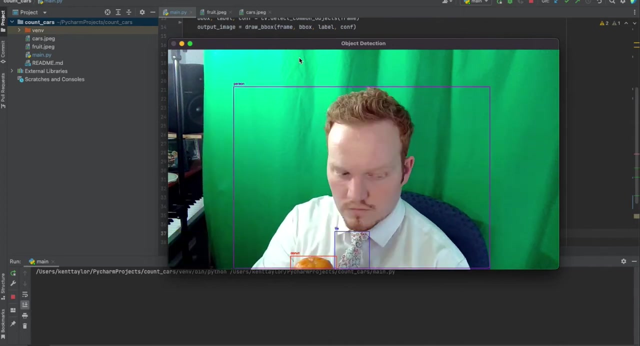 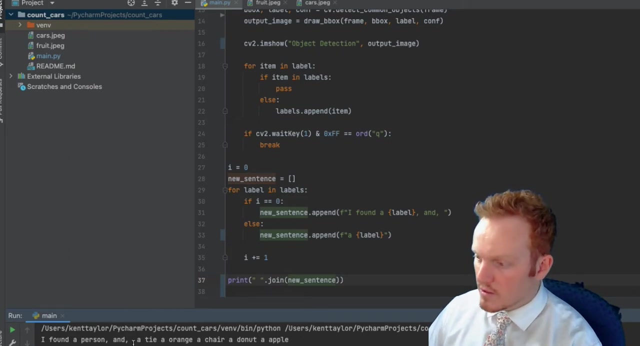 new sentence. So that will turn this list into a string. So let's go ahead and test that out. Perfect. So after hitting run and after it found those two, I'm going to say print space, dot, join, and after it found those things, check it out, It added each of those things to the list. So it said: 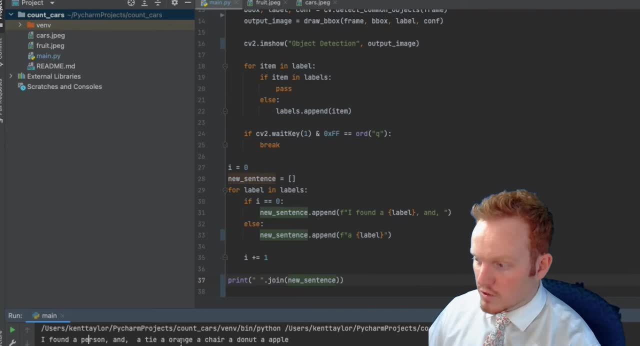 I found a person and a tie orange, a chair, a donut apple. Again, this might look kind of weird with the commas, but it's going to help with the pauses when the computer says it out loud, So very good. If we have that working, just fine, then let's go ahead and add our speech. part of this. 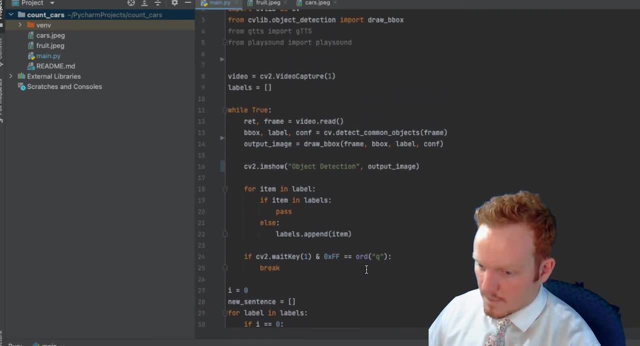 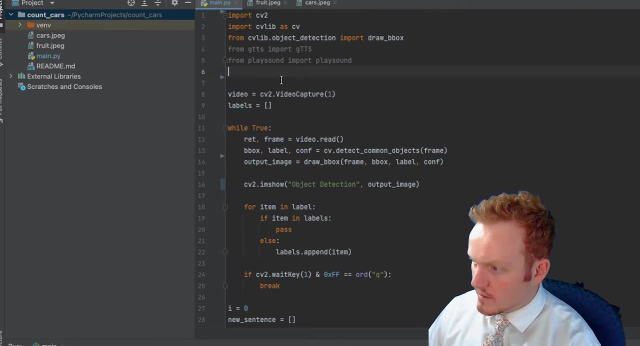 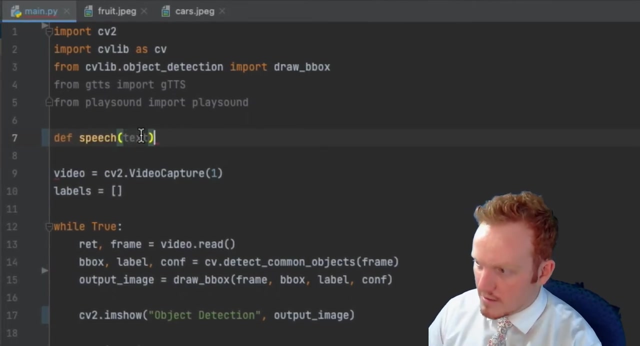 So, towards the top of our project, I'm going to now add our speech. So let's go ahead and define a function. So, def, we'll call this speech And it's going to receive some text. And if you've seen my virtual assistant, where you 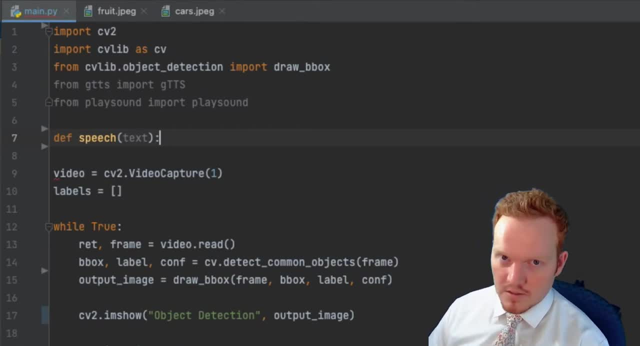 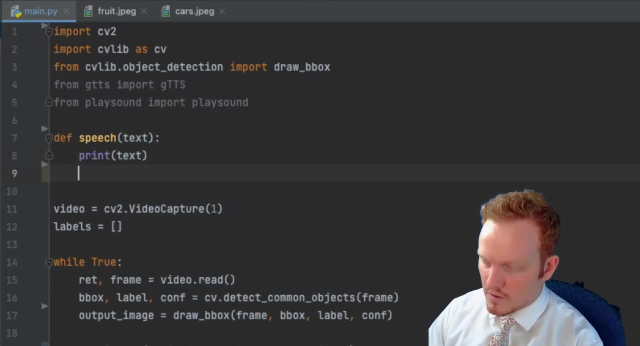 build your own Siri or Alexa. this is the same exact function that we're going to be using. So we're going to say: print that text because we want to be able to see it as well. So we're going to say: print that text because we want to be able to see it as well, And I also want to set my language. 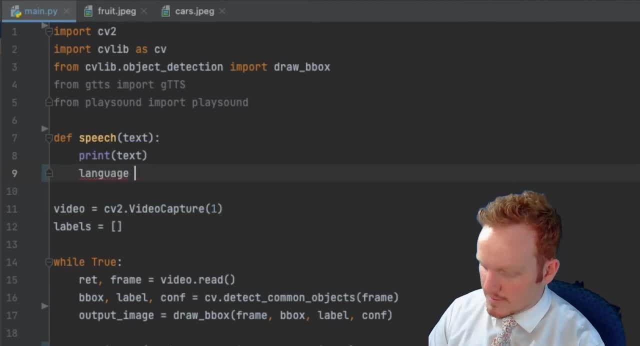 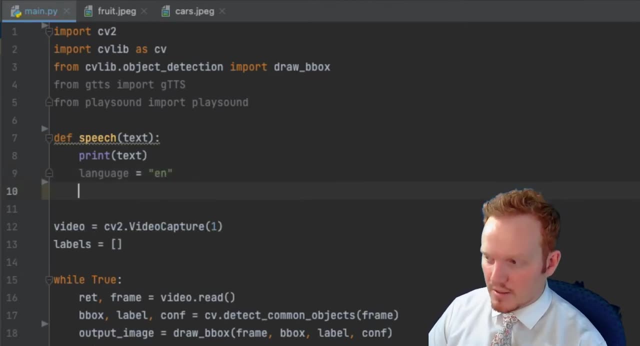 to whatever I want. I'm going to set mine to. we'll call it yeah, we'll say English, So EN. If you want to do Spanish, it's ES or Japanese, it's JA. You can always look those up on Google if you'd. 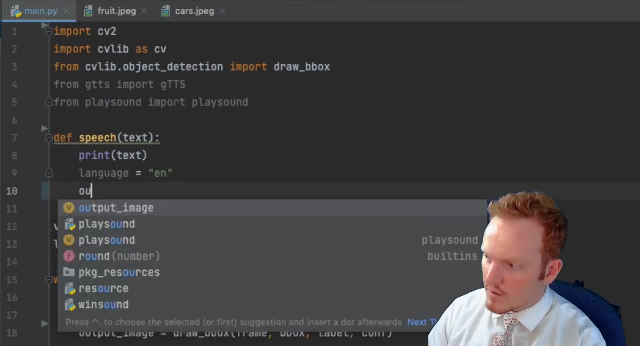 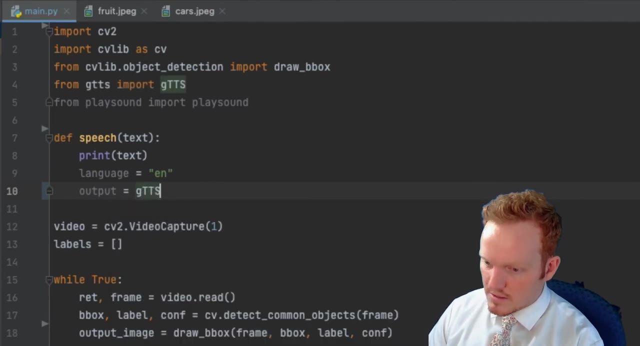 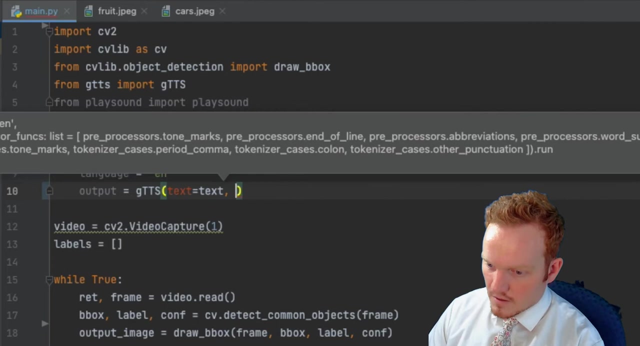 like to, but we'll do English for now And then we'll give this some output. So output equals. now we're going to use GTTS. So GTTS, which takes some text Which is going to be equal to the text that we're going to send it, comma. Now it's looking for the 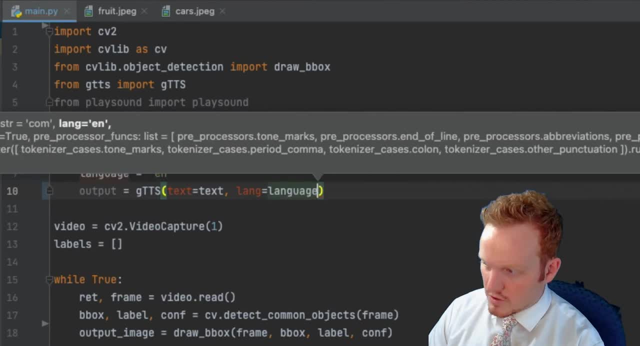 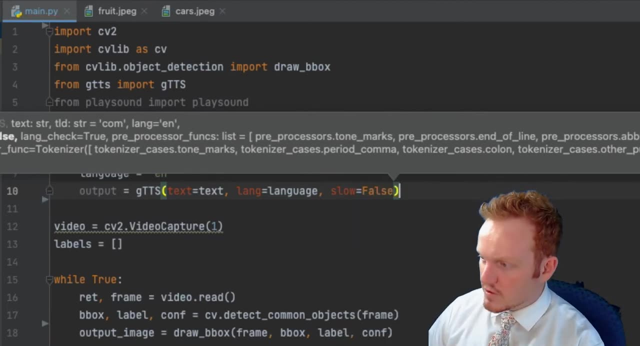 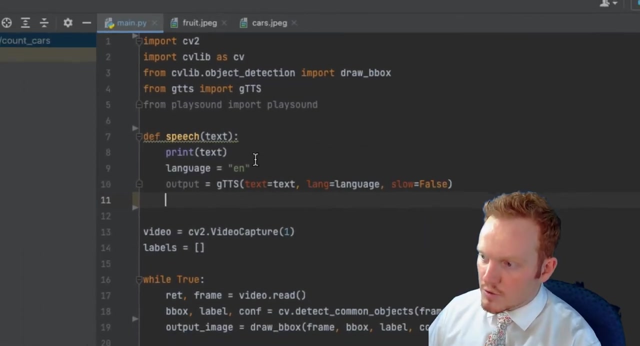 property of language, And so that will be our language. And then, finally, it's going to ask how fast we want to go. So I'm going to say: slow equals false, just like that. Now what we need to do is save the output into a file. So what we need to do is we need to save that audio. 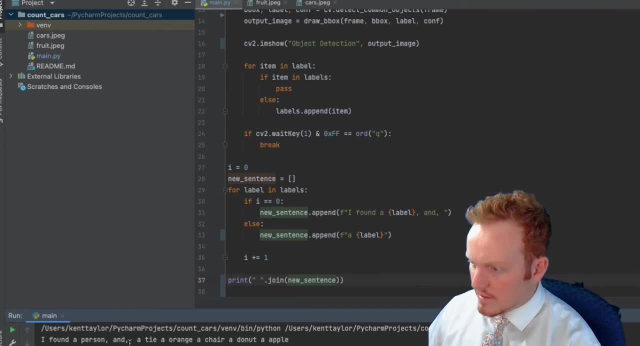 an orange, a chair, a donut, an apple. Again, this might look kind of weird with the commas, but it's going to help with the pauses when the computer says it out loud. So very good, If we have that working just fine, then let's go ahead and add our speech. part of this, So towards the 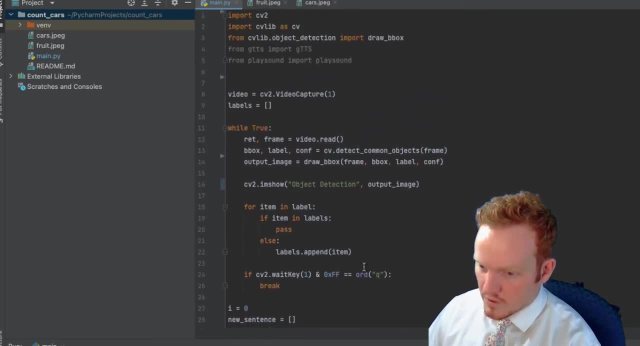 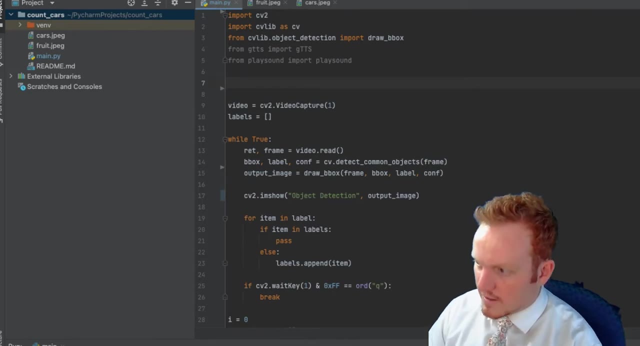 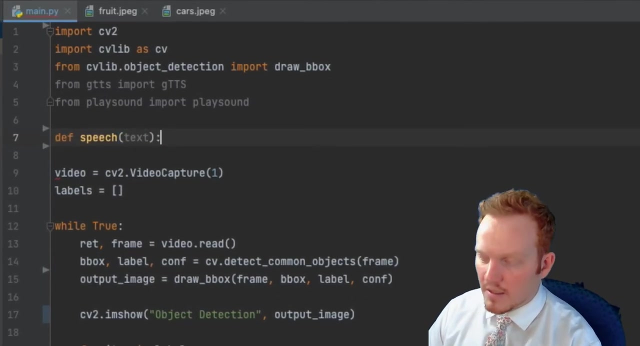 top of our project. I'm going to now add our speech. So let's go ahead and define a function, So def, we'll call this speech and it's going to receive some text. And if you've seen my virtual assistant, where you build your own, 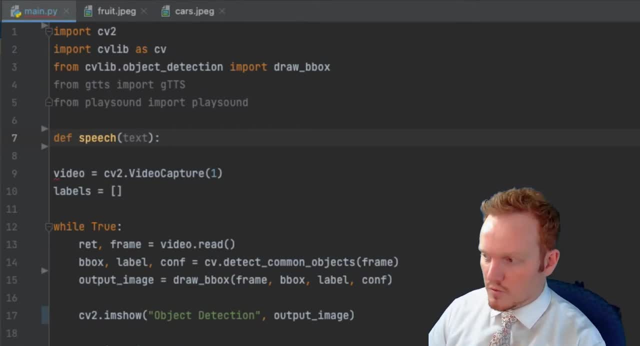 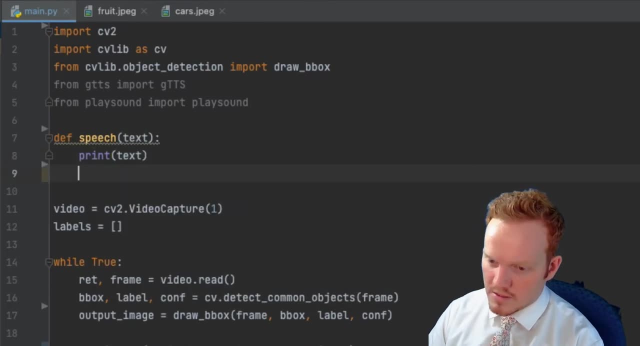 Siri or Alexa. this is the same exact function that we're going to be using. So we're going to say: print that text because we want to be able to see it as well, And I also want to set my language to whatever I want. 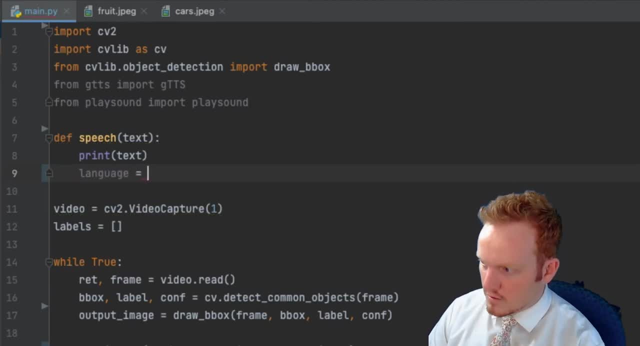 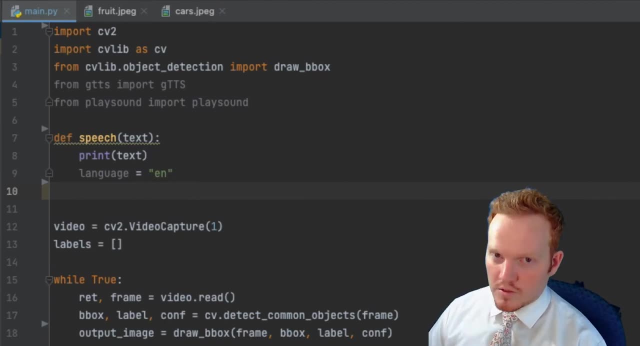 I'm going to set mine to. we'll just call it yeah, we'll say English, So EN. If you want to do Spanish, it's ES or Japanese it's JA. You can always look those up on Google if you'd like to. 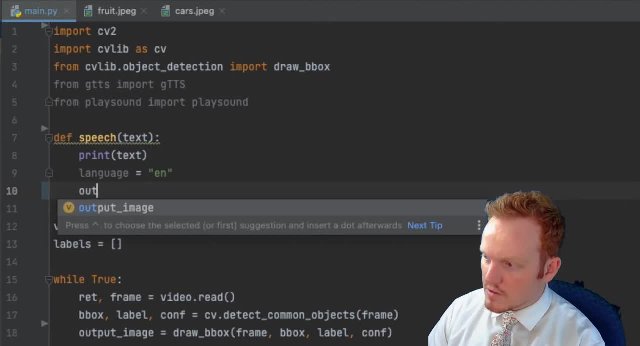 but we'll do English for now And then we'll give this some output, So output equals. now we're going to use GTTS, So GTTS, which takes some text, which is going to be equal to the text that we're. 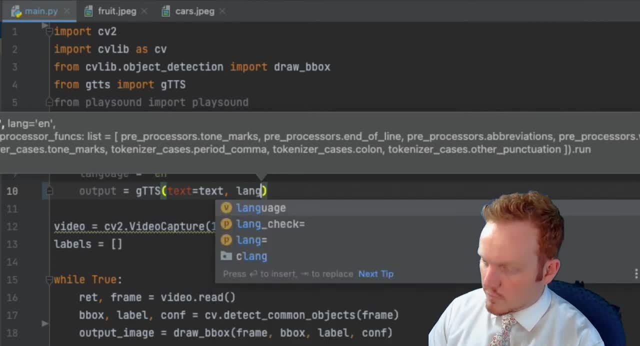 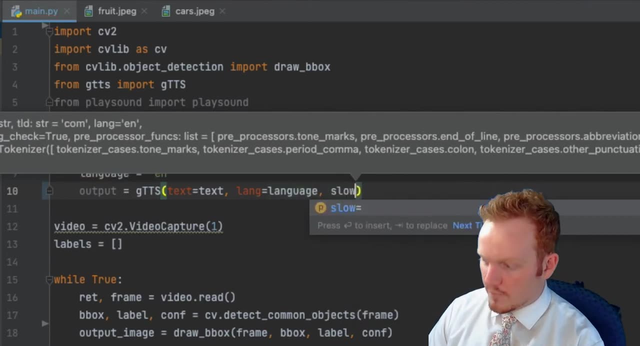 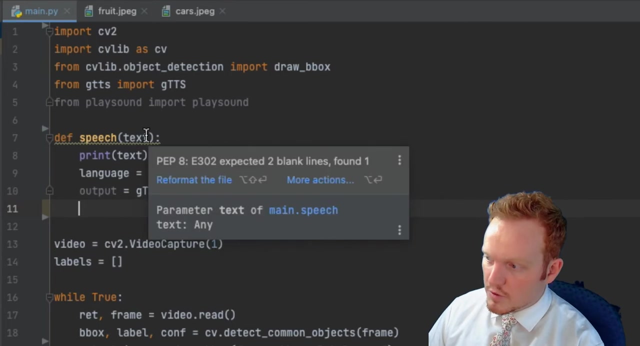 going to send it. Now it's looking for the property of language, And so that will be our language. And then, finally, it's going to ask how fast we want to go. So I'm going to say: slow equals false, just like that. Now what we need to do is save the output into a file. So what we need to do 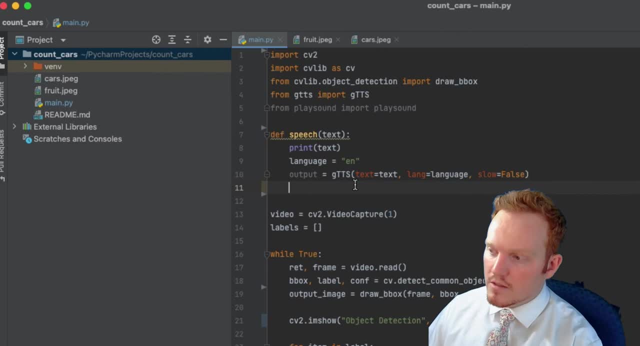 is: we need to save that audio somewhere in our project. So come into your project and let's create a file. So let's say: we want to save that audio somewhere in our project, So come into your project and let's create a new directory And we're just going to call it. 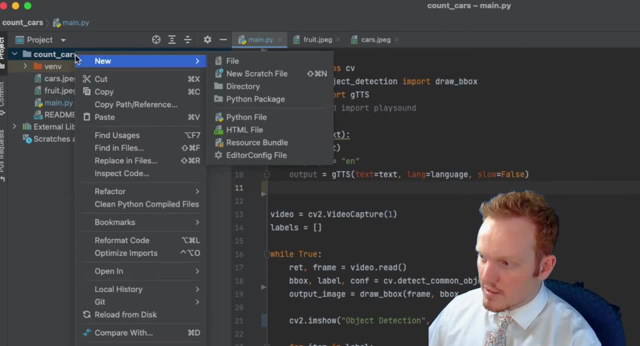 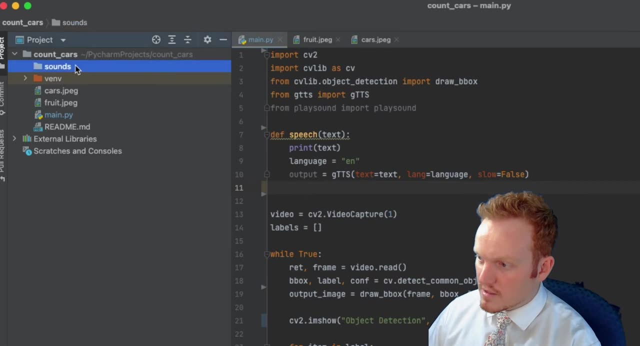 somewhere in our project. So come into your project and let's create a new directory And we're just going to call it sounds. So here's sounds. I forgot to change the name of the project, So don't worry about that, But sounds is just underneath that directory. So with that in place, we can now. 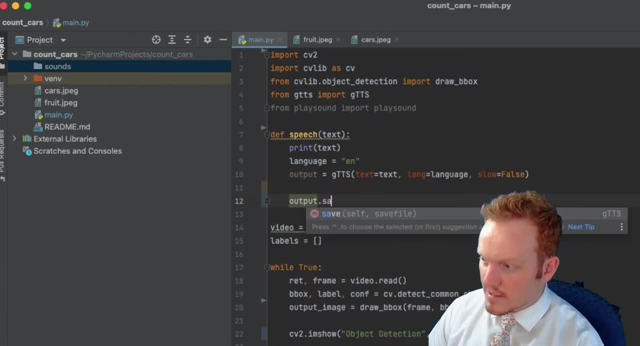 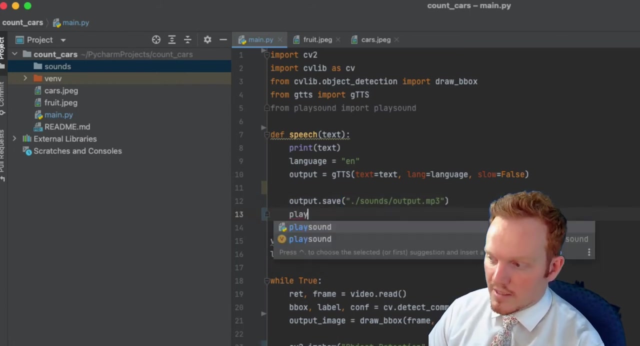 save. So we're going to say output dot- save. Now we're going to tell it where to save. So I'm going to say output dot- slash sounds. And now call your file whatever you want. I'm just going to say output dot- mp3.. So this will be a mp3 file And then, finally, we're going to have it play the. 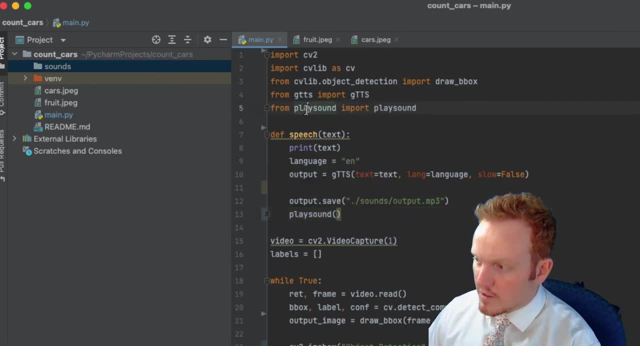 sound. So we're going to use the play sound library that we imported up here And we're going to say play sound, which is going to be that same exact location, output, dot, mp3.. And now we got to send whatever text we want over here. So down here we have a print. Instead of print, I'm going to say: 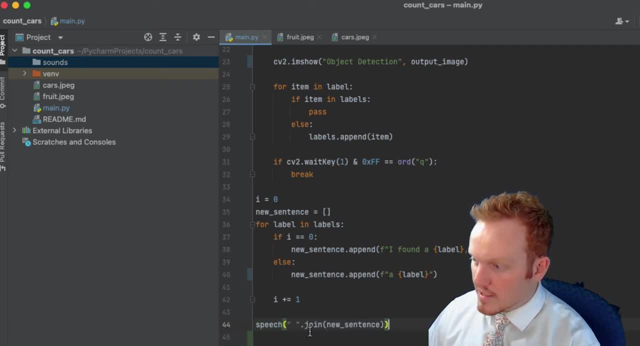 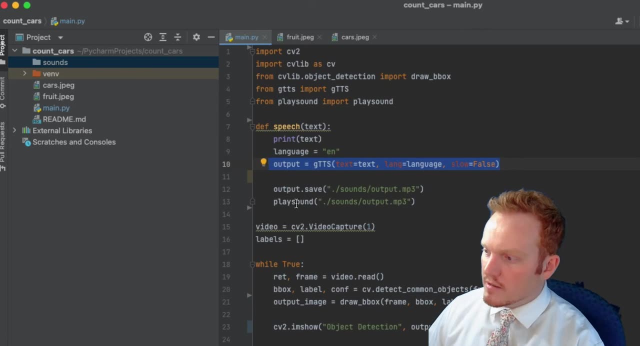 speech, because that's the name of our function. So that will send our string to our function And it's going to take our text and make it into actual speech. It is then saving And then we're going to play that sound. Let's see if this works. 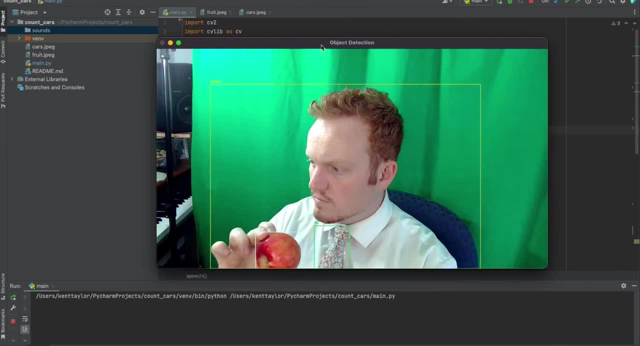 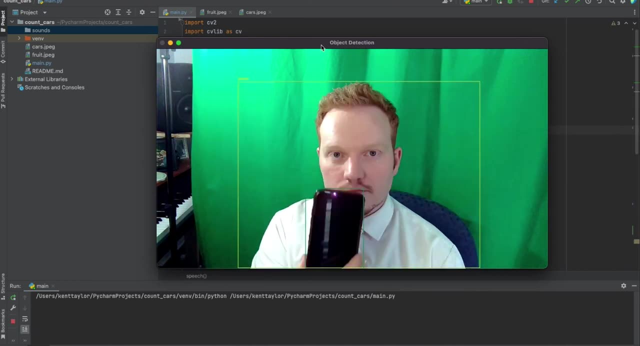 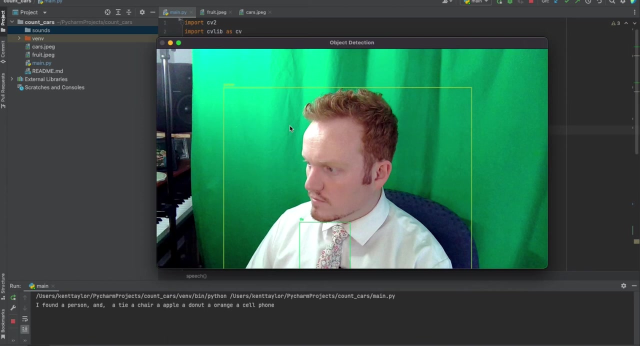 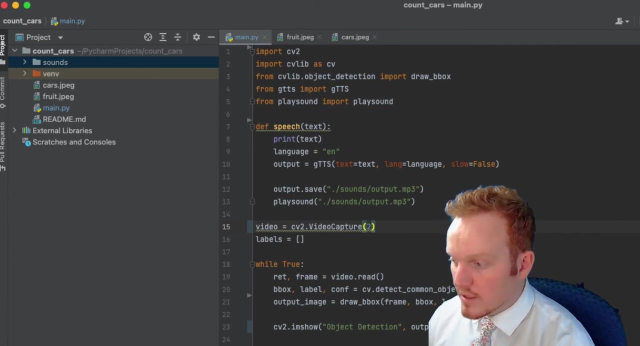 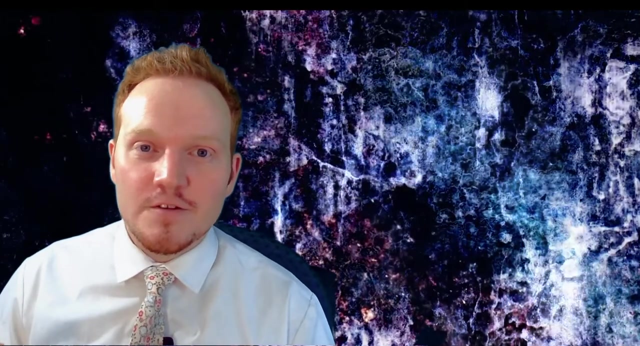 So hopefully you could have heard that. But it did say I found a person and a tie, an apple, orange, a cell phone, So that is working. Great Congratulations if you just accomplished that. That was really cool, pretty simple, And if you. 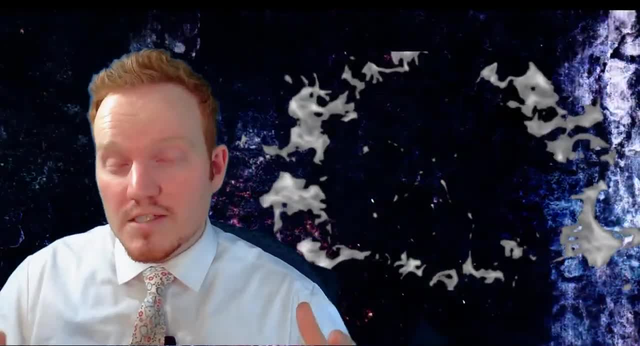 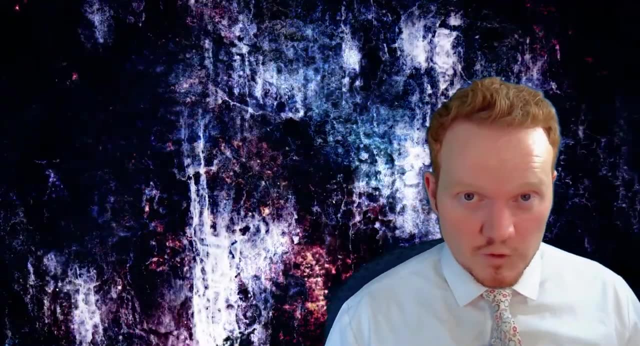 have any questions, please let me know down in the comments. If you have any requests, please let me know. Don't forget to drop a like and subscribe so that you are notified of my next tutorial. Thank you so much and happy coding. You know you're loved. 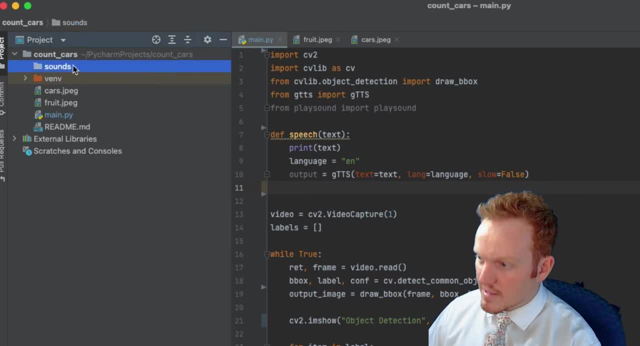 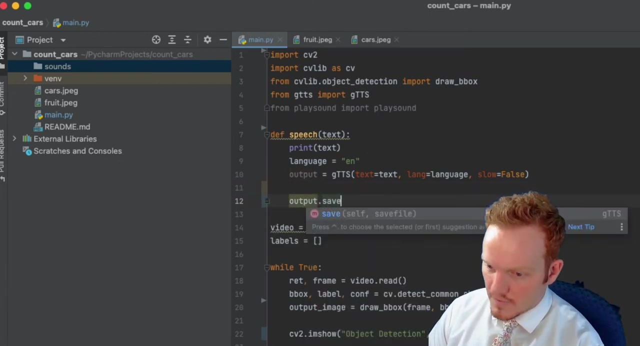 sounds, So here's sounds. I forgot to change the name of the project, So don't worry about that, But sounds is just underneath that directory. So with that in place, we can now save. So we're going to say output dot- save. Now we're going to tell it where to save, So I'm going to say dot.